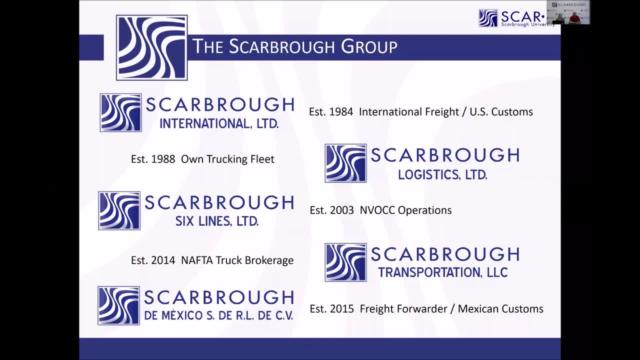 We also have close partners that act as an extension of our team in every major port in the world. We are one of the top US customs brokers in the Midwest and we offer international freight forwarding, domestic truck brokerage, local trucking on our own asset-based trucks, warehousing and distribution. NVOCC services, which is our consolidation division. 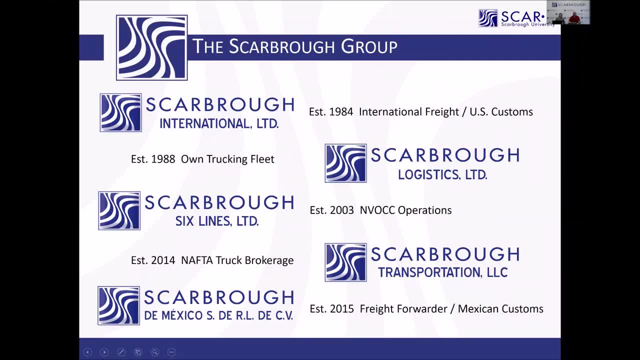 large equipment and oversized cargo moves, NAFTA services, and one of the things we're most known for is our trade compliance consulting and training services. So if you're interested in learning more about us, don't hesitate to call one of us or contact us directly. 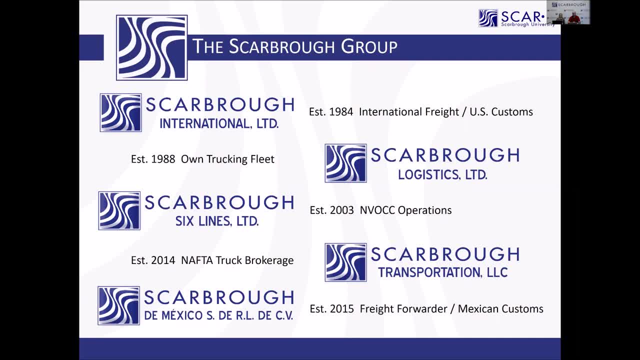 In the next few months, as I mentioned, we'll have a lot of speakers coming up. Some of the speakers we've got joining us include our own Mexico-USA borders operations manager, American shipper. the US Department of Transportation. 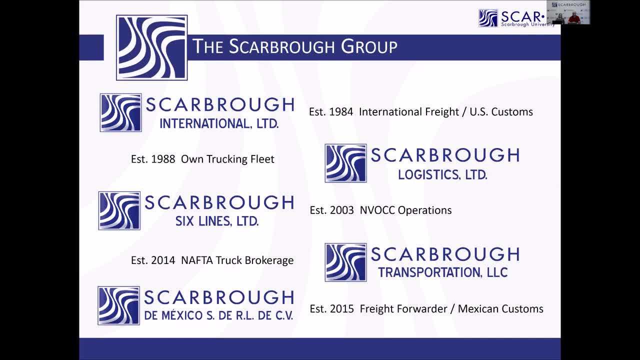 our Canadian customs broker partner, the Export-Import Bank of the United States, among some other experts in Scarborough. So, anyway, stay tuned for more webinars and I'm going to turn it over to you, Kevin. All right, Thank you, Kim. 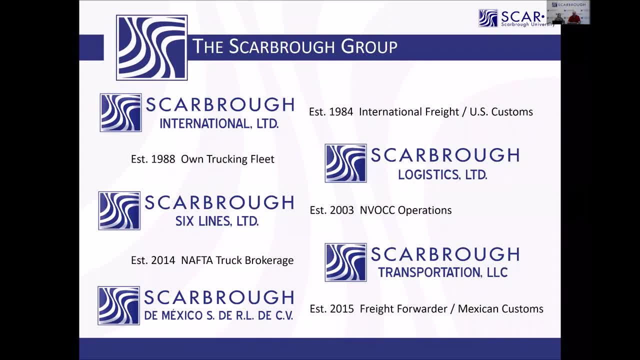 It's great to be back with everybody. Imports is my passion, So many of you that know me know I can talk about different aspects of importation all day long, And here we're going to try to do it in one hour and get to all of your questions. 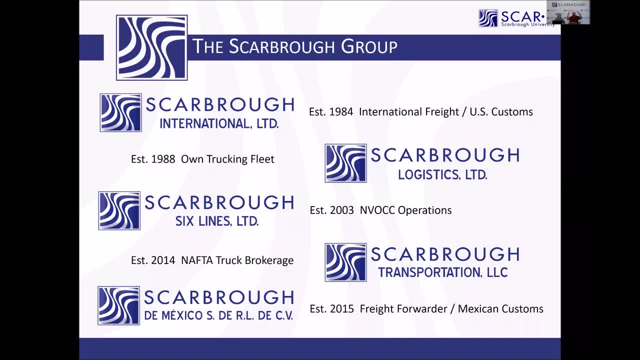 So I'm going to kind of go through this, because we are putting this at a high level, one-on-one. These are some of the basics that folks need to know. Many of you asked some great questions, some great questions. Some of them were very, very specific, very, very specific to specific commodities, trade lanes, those kinds of things. 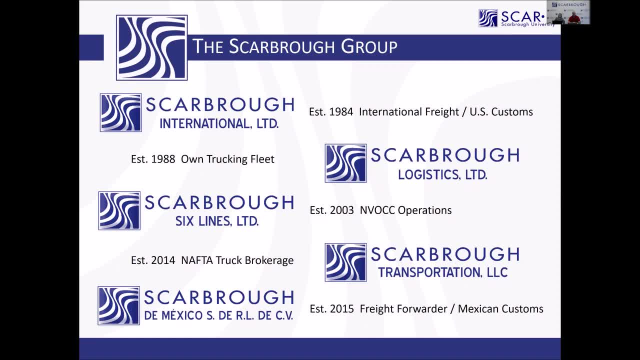 We will try to get to those But, as Kim said, if we can't, then we will get in touch with you on a one-to-one basis, as we have in past webinars for those types of questions, to talk to you specifically. 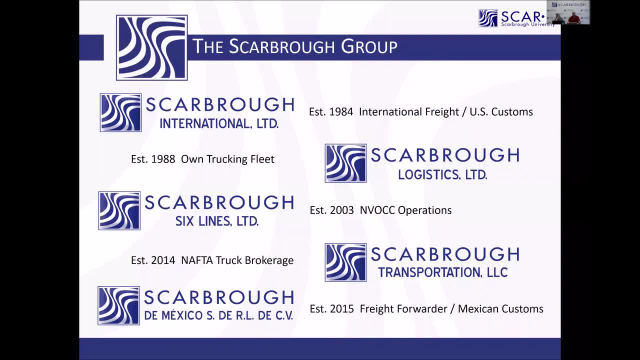 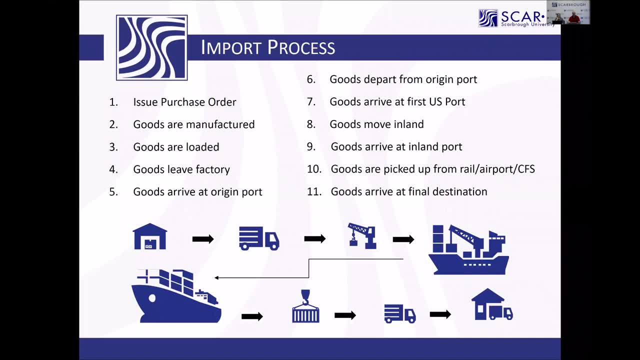 get the details and get you the advice that you need in order to proceed. So today's webinar is Import 101, and we're going to kind of look at this from an import process standpoint. So what I've got showing here is really an import, a very vanilla import process, starting with the issuance of the purchase order to your vendor overseas. 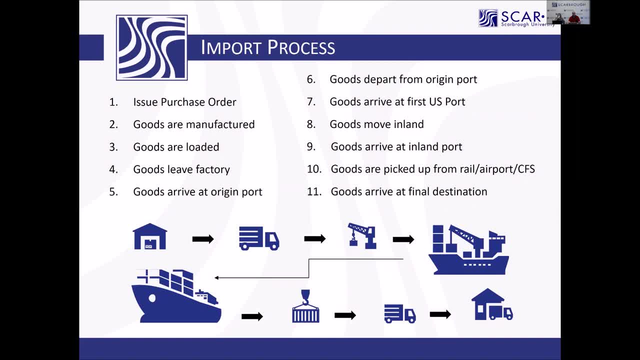 Goods being manufactured by the manufacturer. Goods then gets shipped down to the port, get loaded on board a vessel, a plane, a train, a truck, whatever it might be, depending on the mode of transportation. They leave the factory, heading for the United States. 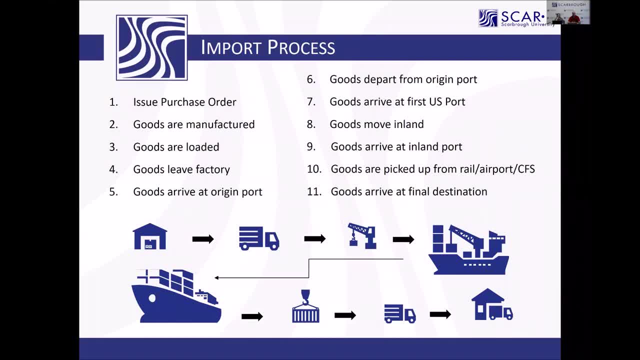 And along the way, we're going to talk about some of the import compliance related issues and things that you need to be thinking about along this process. So, again, this is the process. we're also kind of following you And we're also going to talk about some school logistics that you need to be thinking about along this process. 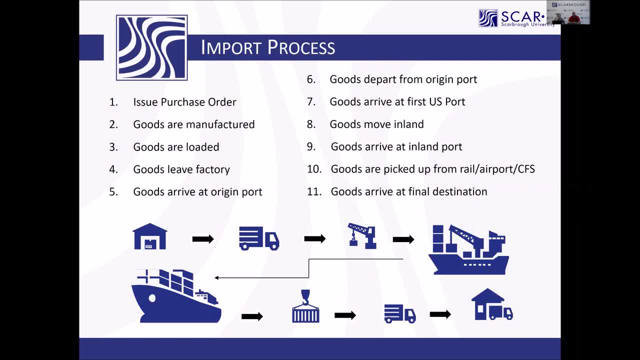 So, again, this is the process. we're kind of going to kind of follow and talk about some things that we want you to discuss before we get to here, things that happen during this. Now we may lean a little bit looking at the group of people that 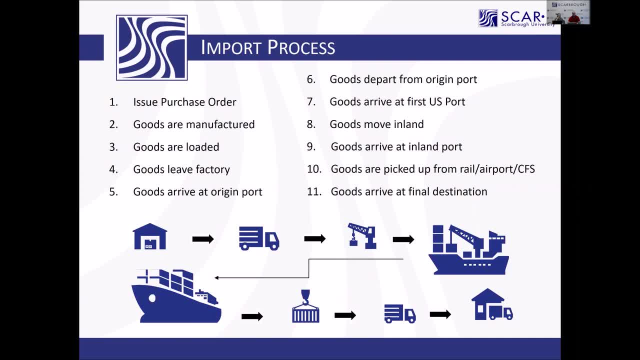 are attending today. We've got a lot of ocean importers here, so we may lean a little bit that way for today's purpose, But anyways, this applies to all modes and we will mention all modes of transportation today. So let's start out with the issuance of the purchase order. This is something 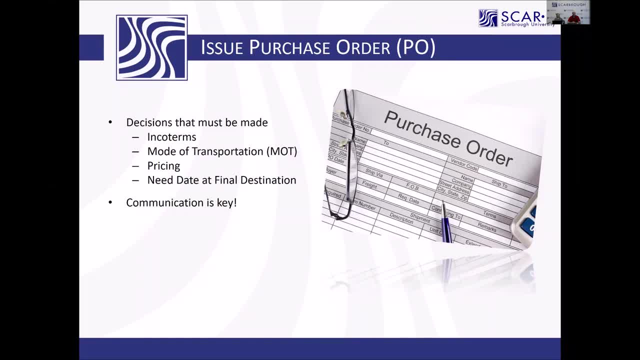 that you do on a daily basis. Many of you are doing this multiple times a day to your overseas vendor. But what are you thinking about when you issue that purchase order- Not just the number of pieces you want and when you need them to be here for your just-in-time manufacturing or your 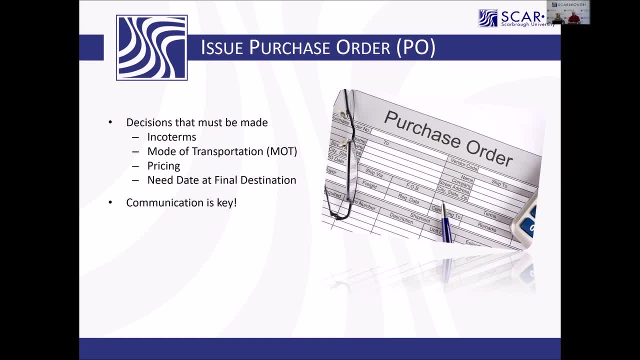 just-in-time distribution services. but things that you need to be thinking of are one: what Incoterm am I going to use? And we're going to focus a little bit about Incoterms here in a second, But Incoterms is a presentation that we could give all on its own because of the 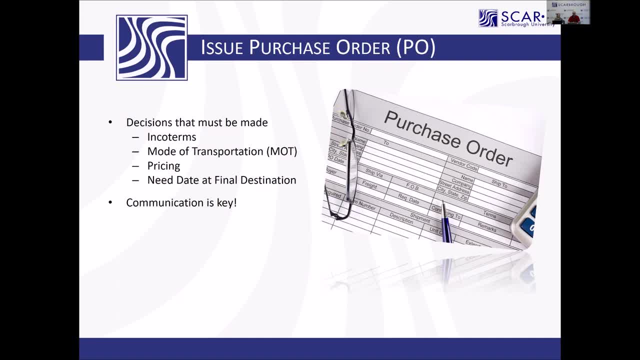 intricacies. I know I give training All over the country to our clients, to the purchasing folks, to the accounting folks, et cetera. as it relates to Incoterms and what Incoterms are And we've got to be thinking of 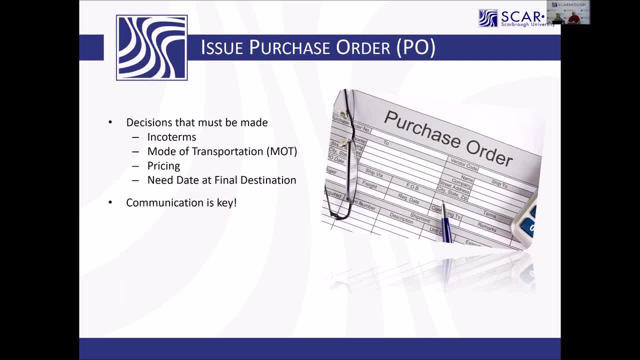 what mode of transportation am I going to use to get the goods from origin vendor to the United States here, along with the pricing to accommodate that that meets that final destination goal? as far as when is it going to get here? So the key in that is again communicating that And as we 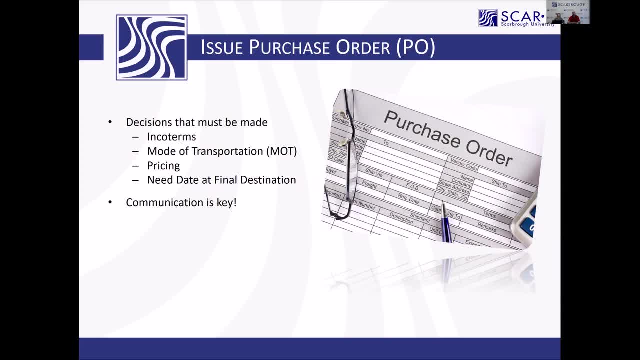 talk through this. we're going to be thinking about what modes of transportation am I going to use? through some of this, be thinking about your purchase order, And does your purchase order provide your vendor with all the information that they need in order to make a successful? 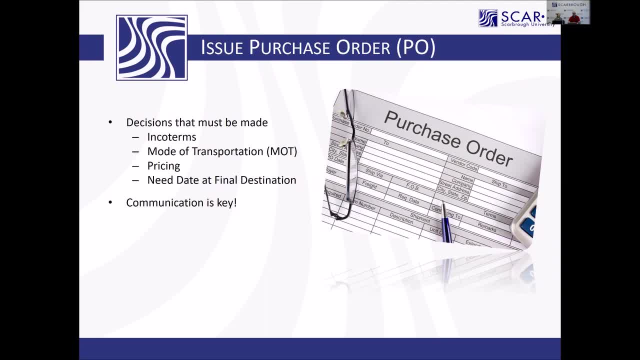 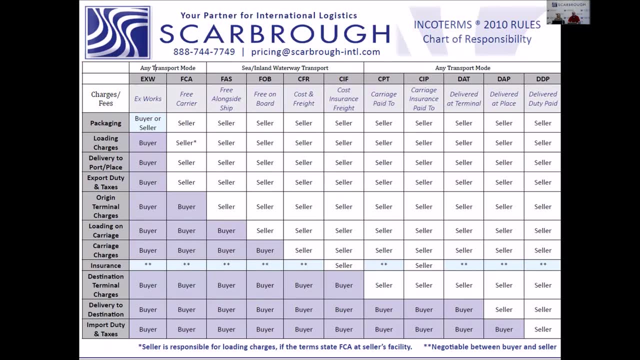 importation for you in the end. So let's talk quickly about Incoterms. I've got up here the Incoterms 2010.. The Incoterms roughly change about every 10 years or so, at least the first book. 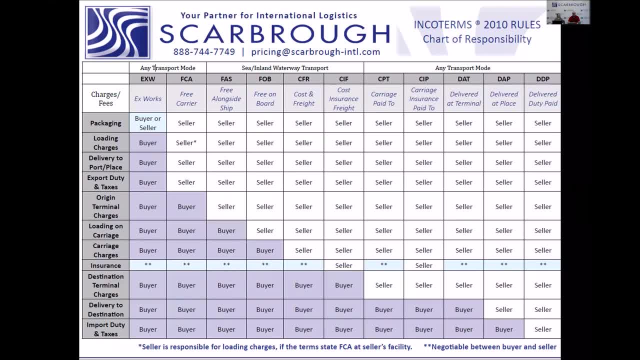 the previous book was in 2000,. this last one in 2010.. And Incoterms tell us two things and two things alike. And Incoterms tell us two things and two things alike. And Incoterms tell us two things and two things alike. They tell us one: where does who pays for what? And the second is: 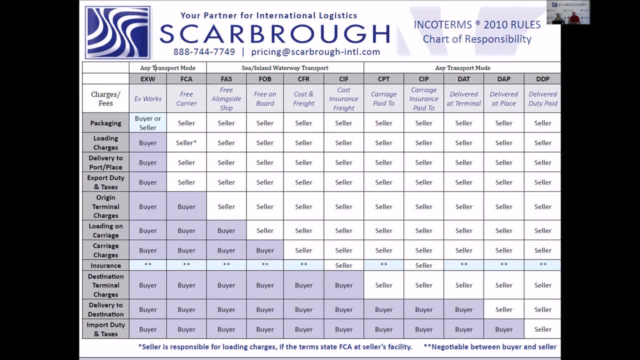 where does risk of loss transfer? That's all Okay. so anybody that tells you that Incoterms might say rumors out. there are things that are falsehoods. that rumor or is that Incoterms tell me who has to be the importer of record? Nope, doesn't tell you who has to be the importer of. 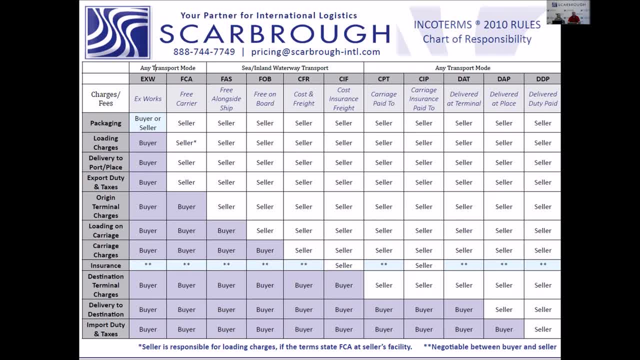 record. It tells you who has to pay for that And it tells you where risk of loss transfers. So that's all Okay. so anybody that tells you that Incoterms might say rumors out there are, transfer happens, Okay. So when I look at Incoterms and my recommendation on the 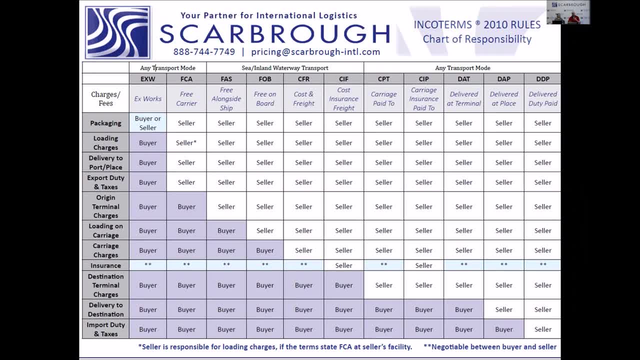 importation side is. it is always an element that Incoterms don't necessarily tell us, but it's control. It's who controls the merchandise. You, as the importer of record. I always recommend that you take full control, And the terms that I use for that are all the F. 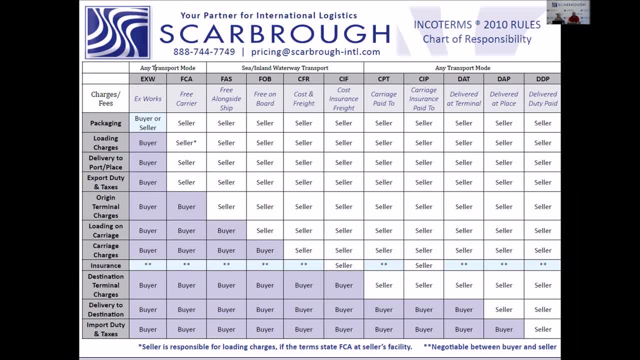 terms. So FCA, FAS, FOB, those are the terms that I recommend utilizing for for you, the importer of record, because they give you maximum control, they allow you to pick which freight forwarder you're going to use And they allow you to control the costs, Because if 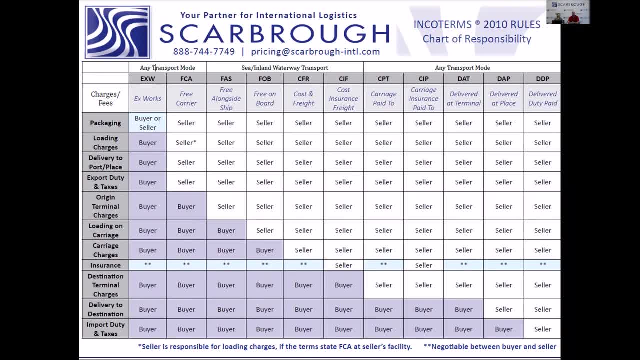 your. if your vendor is utilizing. if you have to use your vendor, straight forwarder odds are pricing changes. your your vendor, especially if it goes down. your vendor is then going to make money and or utilize the freight as a as a revenue string for that, And that's why we recommend that. 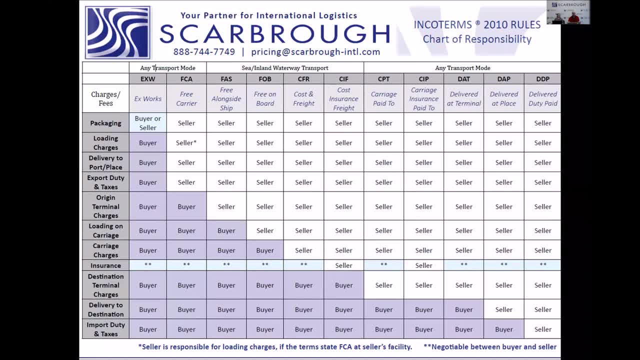 you go with a freight forwarder, you trust You utilize an F term and you take control of that at origin. So, anyways, these terms, Incoterms, are divided up as you can clearly see on. here is one: any mode of transportation. 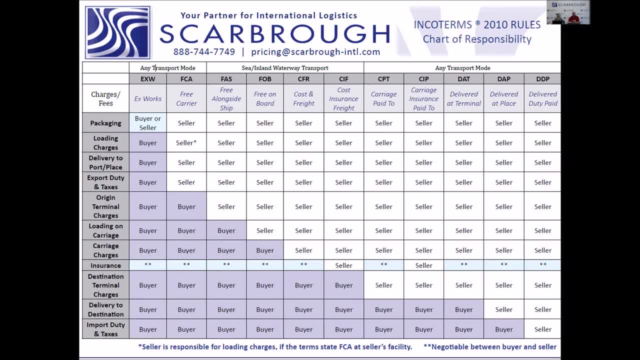 or two: sea and inland waterway transportation And if you look you see FOB right there for sea and waterway transportations. those of you on your call on this call that are sitting behind the cubicle- nobody else can see it, But I want you to raise your hand if you've used FOB for a. 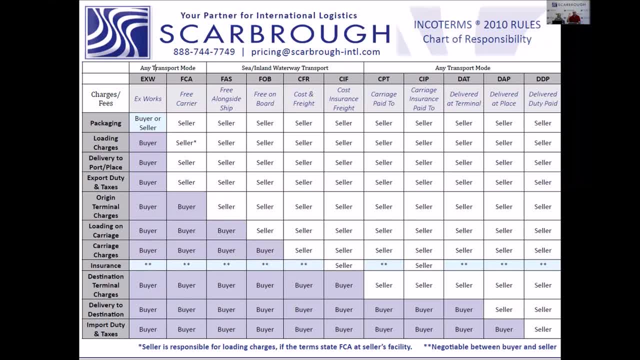 truck shipment or an air shipment, Or even a domestic shipment. Come on, raise your hand. You've done it right By looking at this, at this chart. I would say that you're wrong in doing that. FOB is for sea and inland waterway. 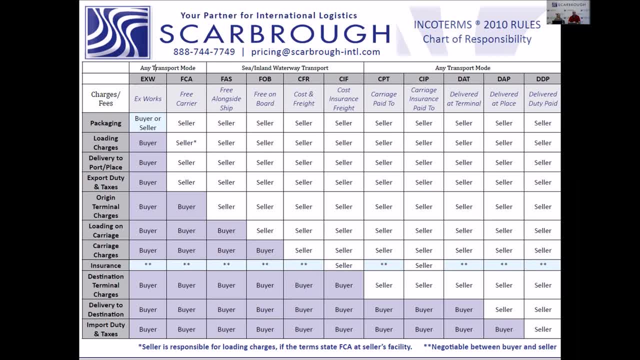 transportation only because it's free on board. free on board a vessel of some sort. So so, anyways, look at some of those any transportation modes. So if you wanted to use FOB, maybe you probably should have used FCA instead. free carriage. 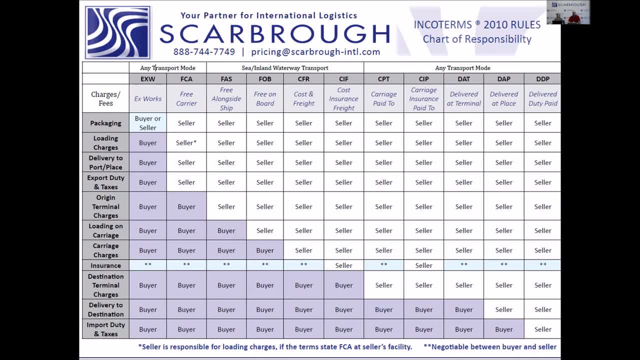 So, but they represent virtually the same thing. It's just that these Incoterms often get utilized incorrectly. But that's the first place to start And if you're interested in presenting Incoterms to your buyers doing training internally, please let us know. We're happy to coordinate and schedule. 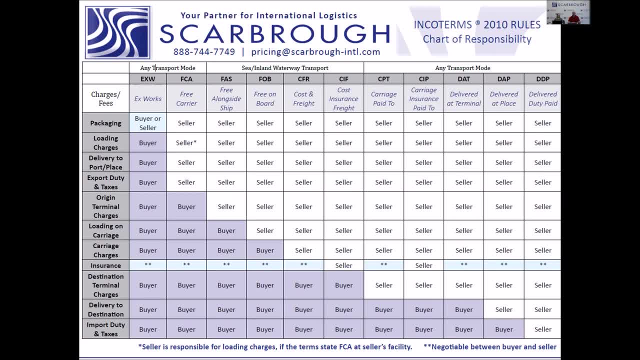 some of that for you, But anyways, Incoterms is number one. It determines where cost transfers and where risk of loss transfers, Meaning that if something bad happens to you, you're going to lose your money, And then you're going to be able to get your money back, And so that's one of the things. that we're going to look at, And then you're going to look at the cost of transportation. So we're going to look at the cost of transportation, which is going to be the most important part of the process, And we're going to look at the cost of transportation. So we're going to look at the cost of transportation And what happens to the 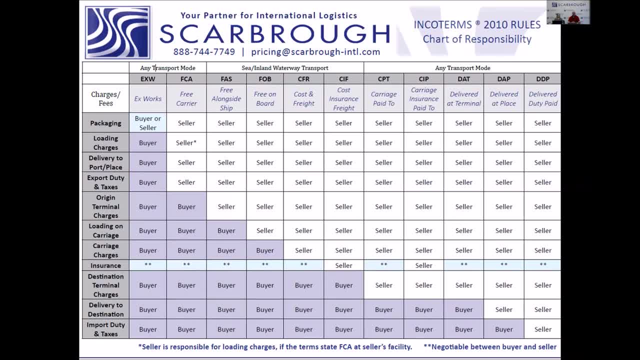 shipment, say it's an ocean shipment and the container falls off the ship. who's who bears that risk And that's what the incoterms tell you. and this chart is a great guide. And again, my recommendation here for the nature of moving through this. 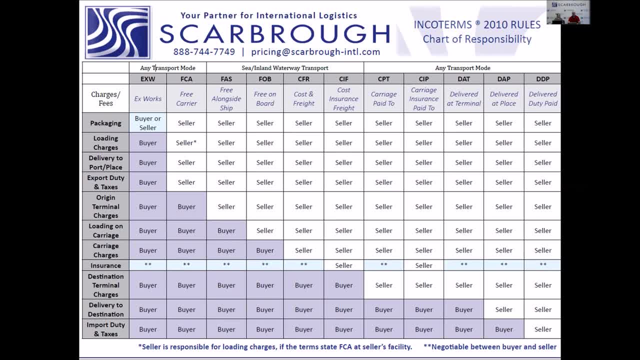 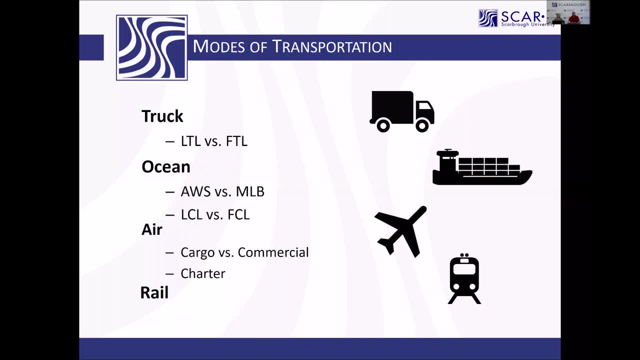 presentation is: is FOB on the import side. On the export side I would recommend a C-turner. So second is mode of transportation. What mode of transportation am I going to select? Okay, If I'm in Canada, Mexico, Ontario is the most reasonable place to pick. to look at the transportation number, Because the transportation number in 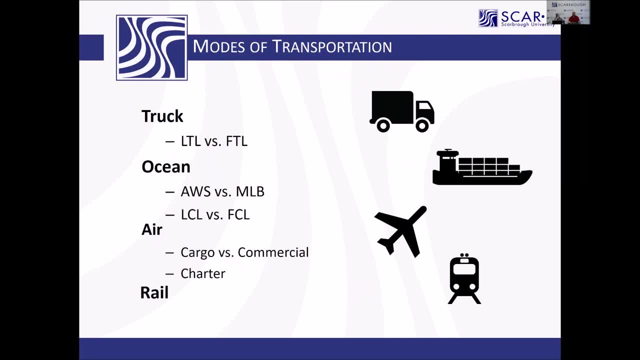 I'm looking, probably a truck or air freight, depending on when I need to get the goods to get here. if I'm shipping anywhere else around the world, I'm probably. I also may be looking at rail from Canada or Mexico, especially for long-haul bulky products rails a great option for that as well, and in, if not. 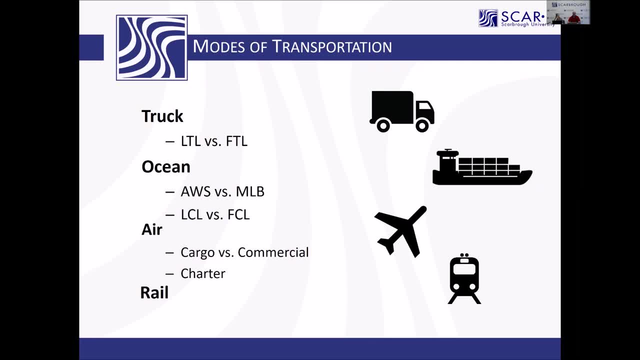 I'm looking at ocean freight, so here we're looking at full containers less than container load for ocean freight. again, the transit time is going to be a little longer with ocean and if you need to get it here quickly then you would go with the air freight. but again, those are the kinds of things that you 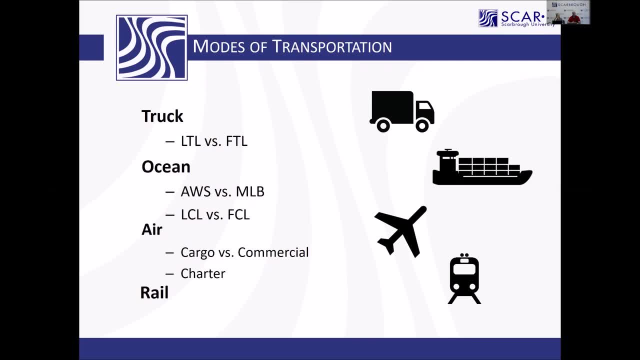 need to determine at the time you issue your purchase orders: when do I need to get it here? because the slower it goes, the less it costs. okay, the slower goes, the less it costs for them for the most part. so look at those options of truck, ocean, air, and well, those are the four modes of transportation. so next steps. 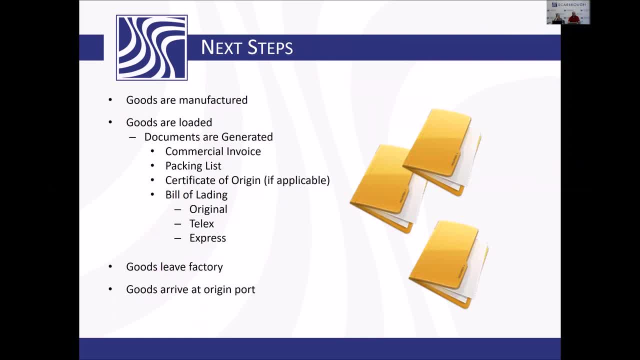 okay, we've issued our purchase order. what happens after that? one good start to become manufactured, right. your vendor overseas is manufacturing the goods that are going to be shipping to you. what happens after that? they? they determine again if you're using an FOB term they're contacting with with our partner overseas or the partner of the. 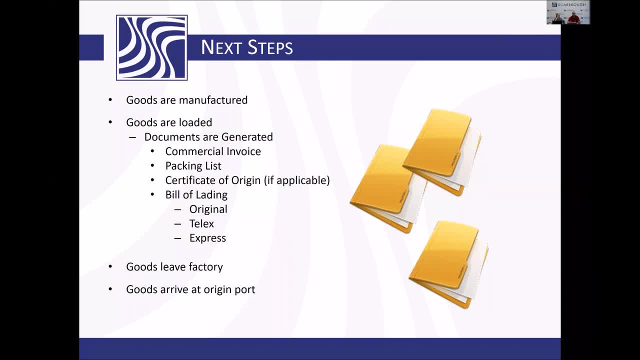 freight forwarder overseas to schedule the, to schedule the shipment to be booked on board a vessel: on board a plane if it's if it's an overseas shipment, and or on truck if it's a Canada, Mexico or potentially, like I said. well, what happens at that time? documents are. 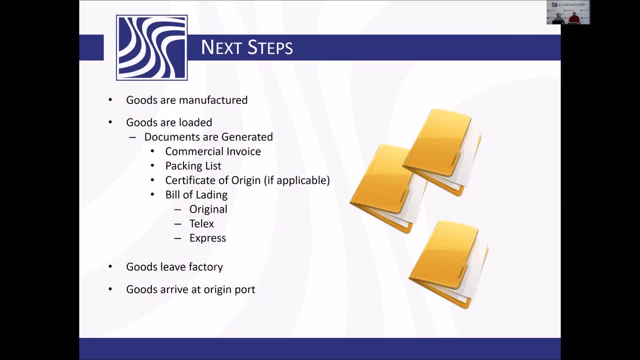 generated vendor is going to generate a commercial invoice, packing lists, certificate of origin, potentially bill of lading. these are all required entry documents as well. so at the time that they're producing these documents, we always recommend that they send these documents to, to, to us, to Scarborough, to. 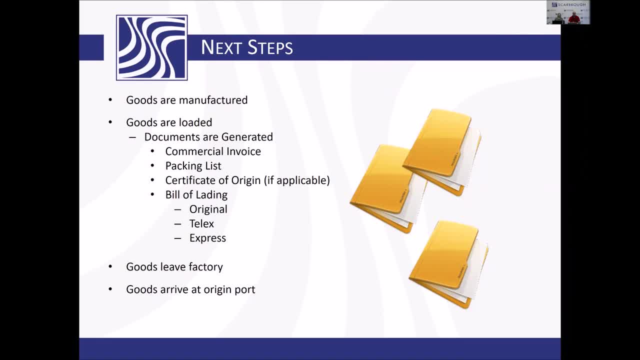 the freight forwarder to the customs broker as well. when I look at one of the documents, the bill of lading- there's typically three types of bills of ladings there, especially ocean freight. primarily I'm talking because bill of lading is title to the goods, meaning that the person 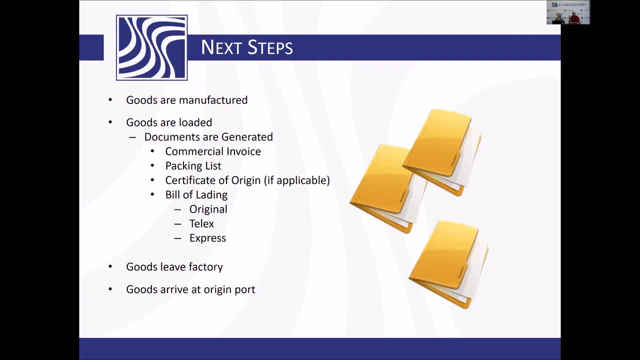 that possesses the original bills of ladings actually has title to those goods. there's one is the original meaning, just that you have the original bill. I can tender that original bill to the freight forwarder and steamship companies and in us take possession of my goods and typically that original. 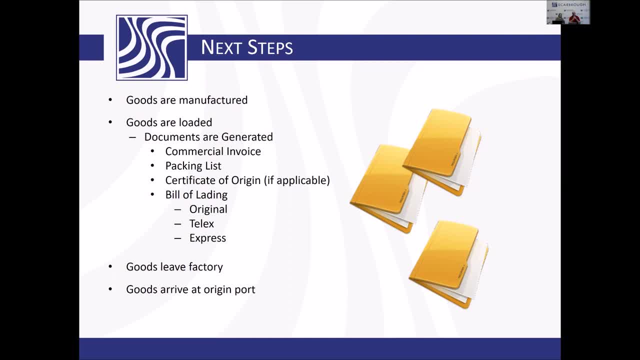 bill of lading isn't sent to you, the importer, until you've met your financial responsibilities or obligations, So meaning that you've paid them and or you're on credit terms with them, et cetera, et cetera. Next is a TELEX release. In a TELEX release, that's a TELEX bill of lading. 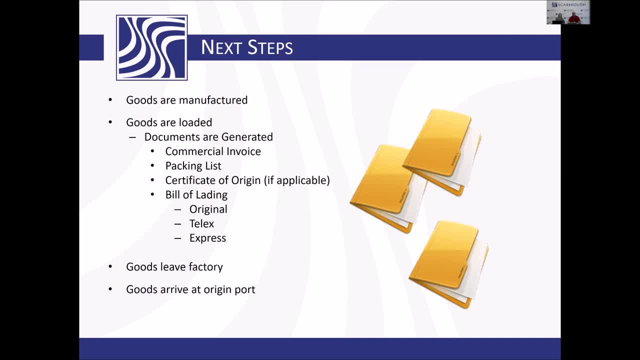 the overseas vendor, for you will receive an original bill of lading. They will endorse the bill of lading and surrender it back to the freight forwarder overseas. What that does is then that freight forwarder overseas will notify someone like myself or the corresponding agent. 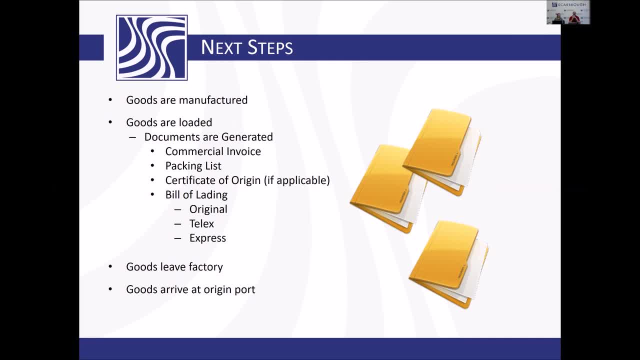 here in the United States that the shipment has been released. What that does is it saves a little time. It saves them from having to end expense from sending it on a courier over to us here in the United States so that you can tender that original bill of lading here. The next is a. 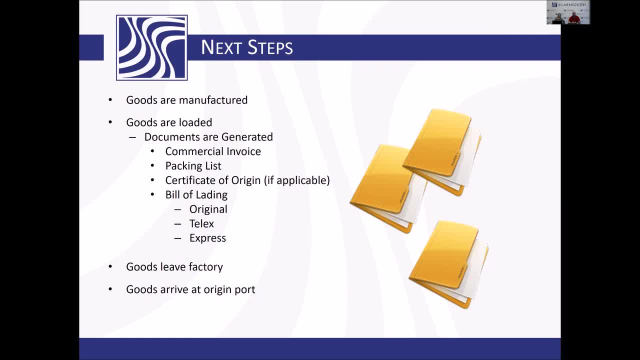 waybill or an express bill of lading. Typically this happens with vendors And consignees that are on terms- credit terms meaning that no original bill is required The minute this shipment, this bill of lading is generated. the person here in the United States. 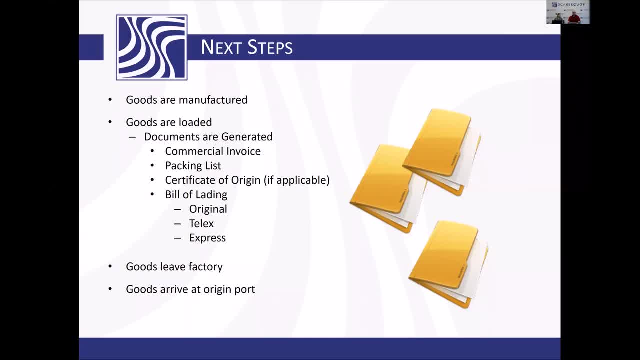 can take possession of it. So if you've got a great relationship with your vendors overseas, we recommend trying to get them to issue waybills or express bills of lading so that there is no original that has to be sent from one person, one party to the next. 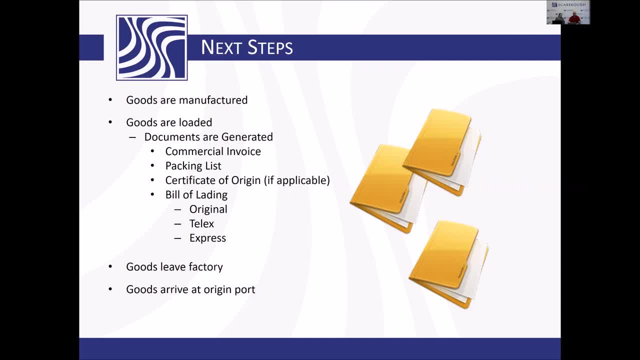 So can I interrupt? If we're a new importer and it's possible for us to request a certain type of bill of lading, what type of bill of lading do you recommend that we request? An original or a telex, If I'm a first-time importer? 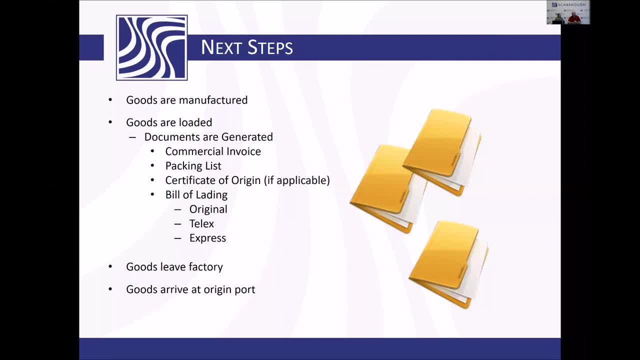 First time or a couple shipments a year. Well, again for that kind of importer, you're probably not going to be on terms with your credit terms with your factory or your manufacturer overseas. So they're probably going to want to issue an original bill of lading because 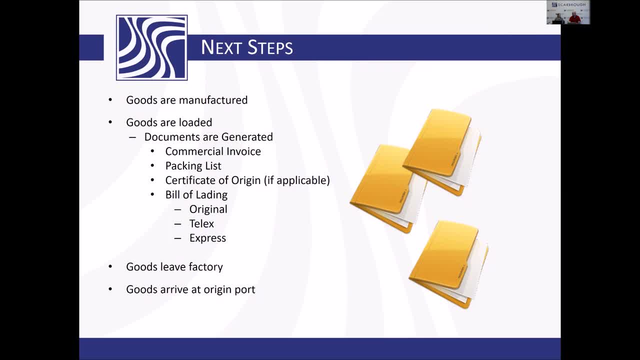 again, they don't want you to just have possession of the goods without payment, And so probably the original would be the way to go. So in that instance they can still ship the goods, Goods can be moving, but you can't get possession until you tender that original bill of lading. 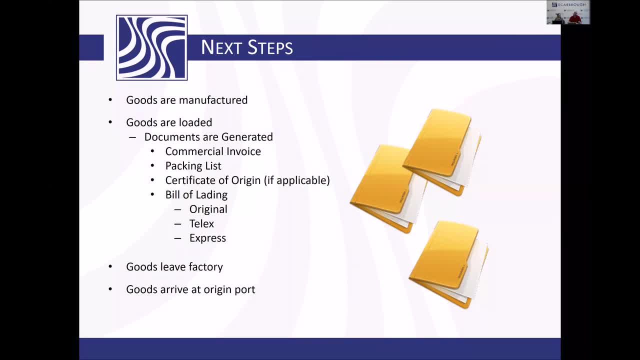 So that's probably the situation that you're going to be in, especially if you're a first-time importer and or you don't import a lot, so to speak. So anyways, that was a great question. So next what happens is, again, goods are loaded, they leave the factory. Again, if it's an ocean. 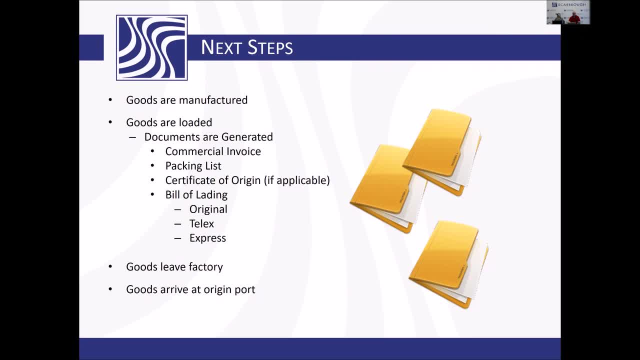 shipment, overseas, or even an air shipment. those goods are going to load it in a truck and they're going to get taken to the port, either to the airport or to the seaport, to be loaded onto a container- If it's less than container- and or loading leaving the factory. it could have been. 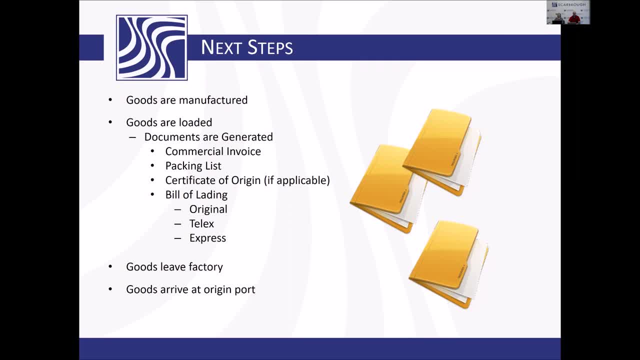 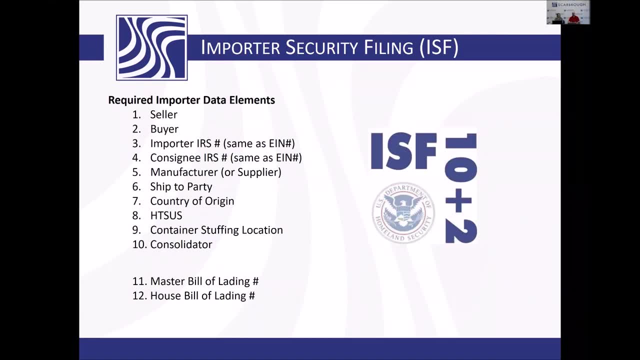 loaded inside a full container. at that point It's going to arrive at the origin port overseas, And at that point a couple things happen. One is: um, the manifest from the freight forwarding company is typically being surrendered to US Customs here, meaning that we're going to transmit what manifest information is, And 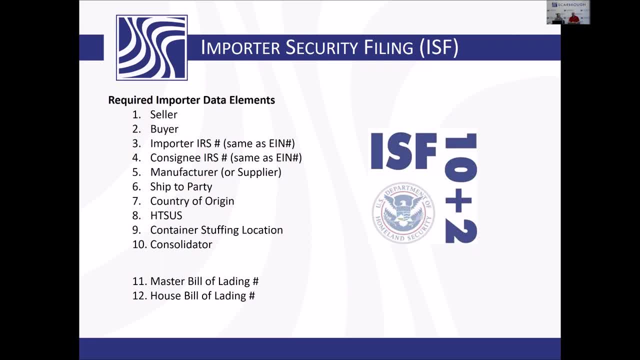 second is is that the importer security filing deadline is starting And that deadline for the importer security filing is 24 hours prior to the loading of the vessel by law. Okay, Now I will give you a little secret. here is that the steamship lines currently don't transmit the date. 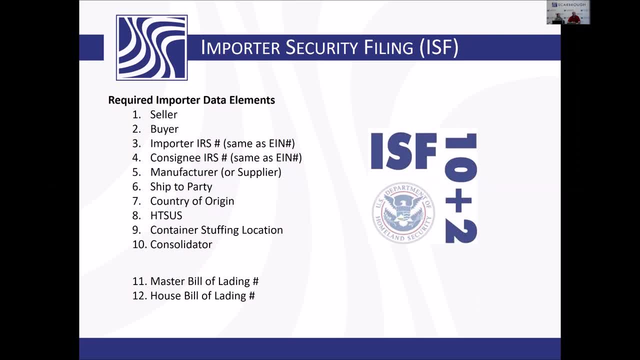 that it's contained in theual order. The ship is going to be loaded into the port, but it's not or is loaded, so customs is measuring the loading actually based on the day that it's leaving, so it actually gives you a little more time, typically at scarborough. we recommend that. 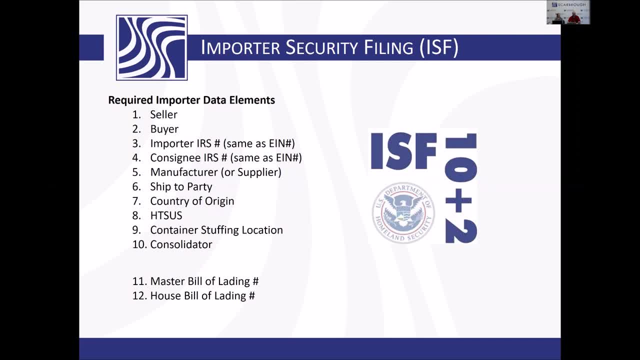 we get this information 48 to 72 hours in advance or at the time that the shipment is being loaded. if we could get it at the time that the shipment is being loaded, that's great, because we can transmit the security filing to us customs as far in advance as as need be. and these are the 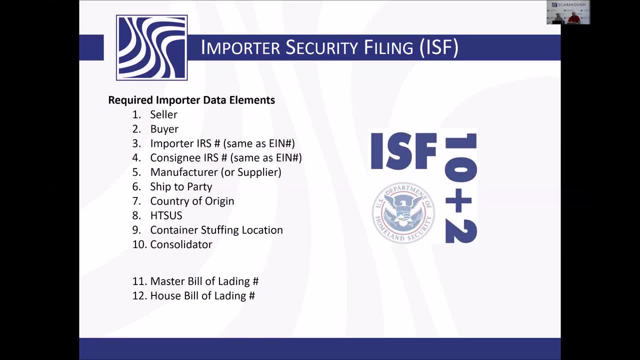 elements that are required from the, from your vendor. we need to know the seller's name and address, the buyer's name and address. we need to have your importer ein number which, if we're the customs broker that's transmitting that, we've already got that, so you don't need to give that. 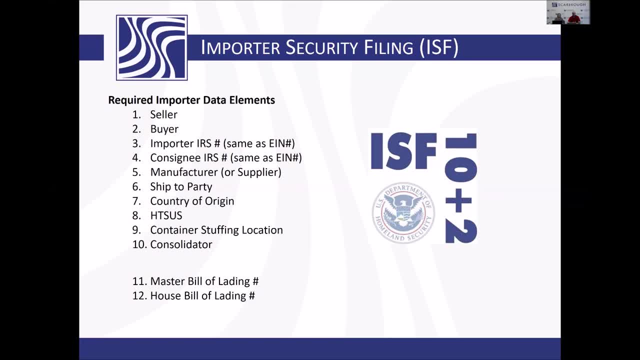 to your vendor overseas to put on their documents. so again that importer ein number, irs number, don't, don't have them put that. don't put that on a purchase order, um. your customs broker has that on file. it was required on the power of attorney, um when you signed. 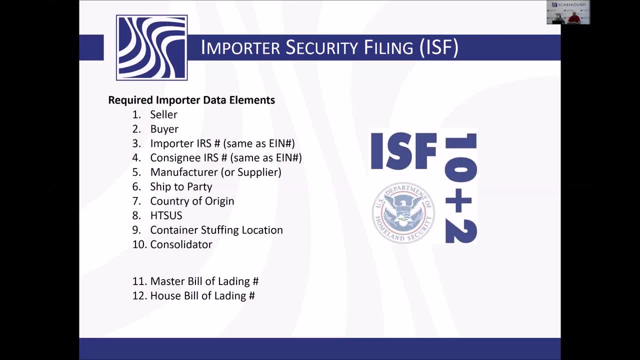 one of those documents. so we need to know the seller's name and address, we need to know the one for customs broker to handle your import clearances and we need to know the manufacturer or supplier- and again that may be different than the seller of the goods- the ship two party in the 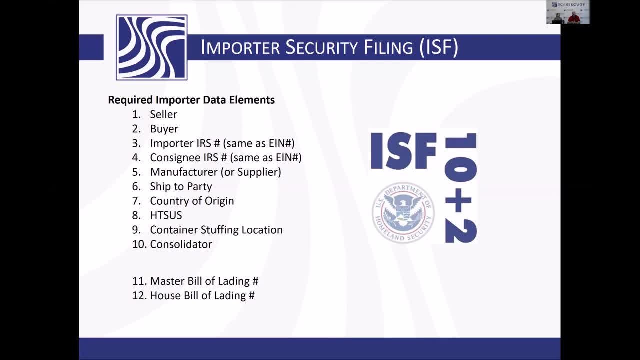 united states, the country of origin, the harmonized tariff number to a six digit level. a harmonized tariff number is 10 digits, but we'll we'll talk about that here in a minute- um, the container stuffing location and the consolidator. those are the 10 elements that are required for us to 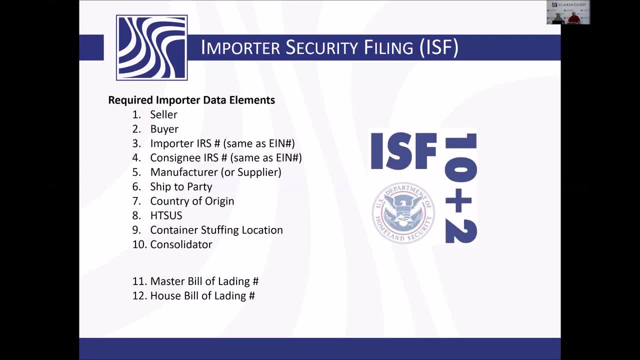 transmit to customs. and then the steamship company actually transmits 11 and 12 element there, the master bill of lading and house bill of lading. so anyways, at the time your shipment is being loaded overseas, we want to be asking them for the isf information or the importer security filing information. um timing again on that. 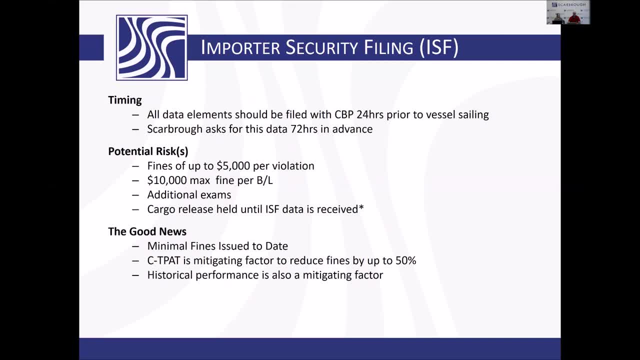 we were asking for 72 hours in advance. what is the potential risk if you don't file it on time? um, one finds up to five thousand dollars per violation and the second is up to ten thousand dollars per violation, and the second is up to ten thousand dollars per violation and the second is. 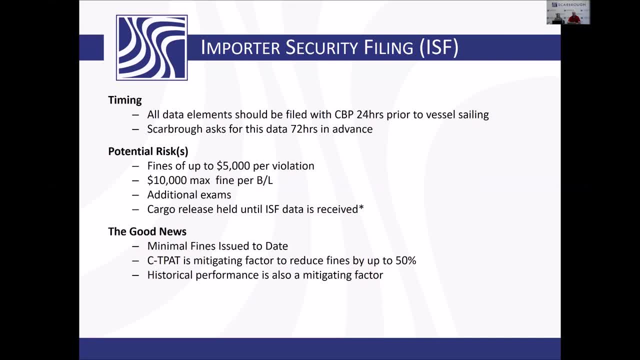 max per bill of lading. it could also generate exams and holds and or cargo releases held at the isf. data is not received um. and why the different levels or um listed here for for potential violations? and i'll tell you. one of them is that for some companies like general motors and some 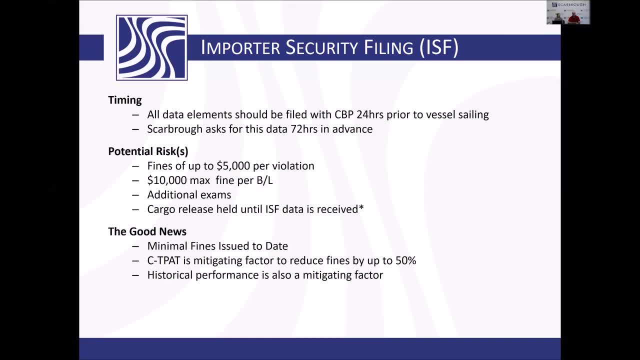 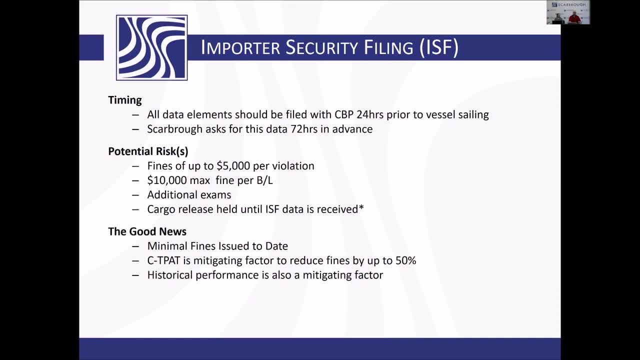 on the line and that line shuts down, that assembly line shuts down, it could cost them a million dollars a day. so having that potential risk- be holding the freight, holding the cargo, delaying it somehow, is oftentimes a larger penalty than than some of these violations. but anyways, customs. 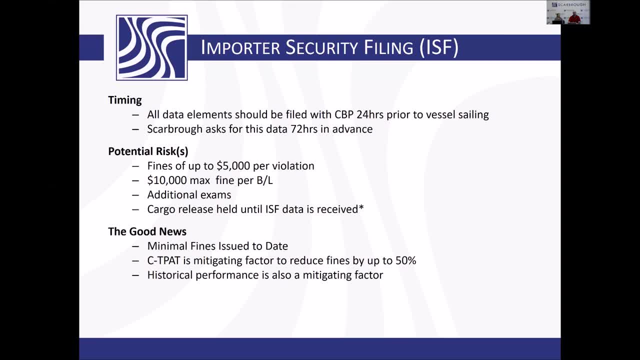 is measuring that violation based on loading date or the date that it leaves. so we've been- we've uh been pretty successful in getting security filings for our clients, and most of the import trade is very good at providing this information today, because this import security filing actually 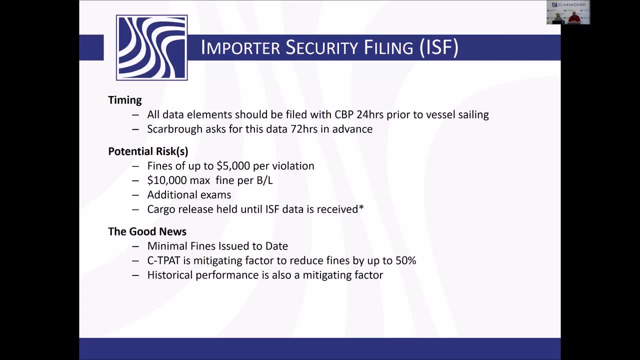 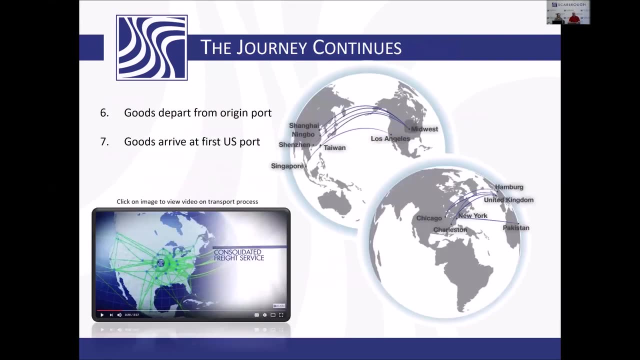 started in 2009.. So, anyways, pretty good at getting this information with regards to that. And again, it's just all about risk. It's all about protecting the borders is what the security filing is about. So now let's talk about the goods. get loaded on board. Say it's on board a vessel. 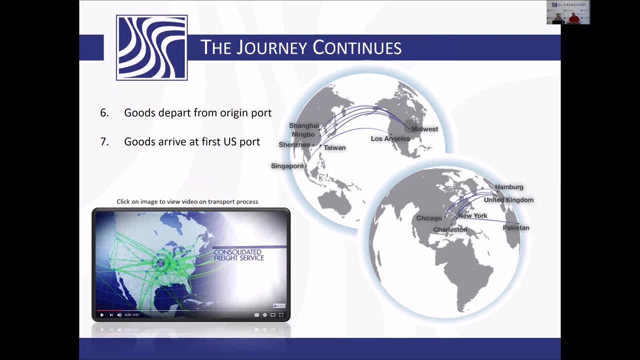 or a plane in that journey before it arrives here. So typically, from a freight forwarding standpoint, you're going to get a lot of information as to when something is going to leave. Okay, you're going to get an estimated time of departure. you can even- we can even- acquire the 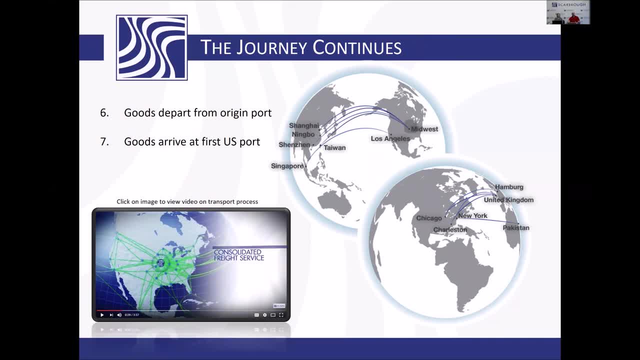 actual date that it left And then we're going to get an actual time that it's going to arrive in the United States. Up until that, especially if it's ocean, there's not a lot of updated information that you're going to get in that time period. 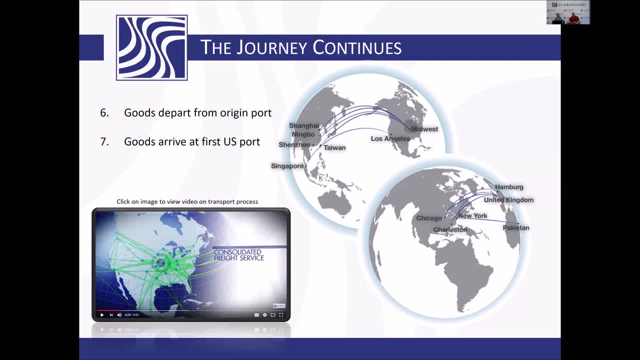 So if you're shipping ocean, just expect that that there might be a lag there. So say it's coming from Shanghai to LA and then moving into Canada or docking in LA. you know that's roughly 14 days. Okay, freight forwarders, we can provide you that information all day long. as far as when? 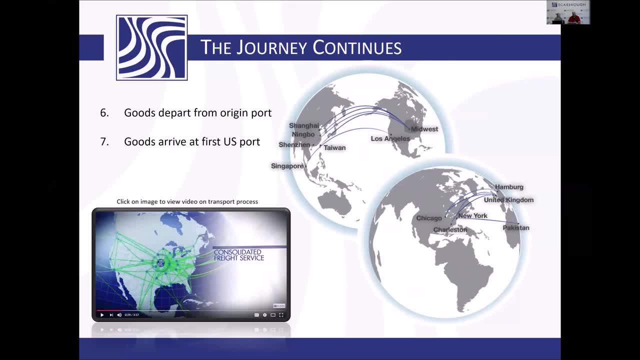 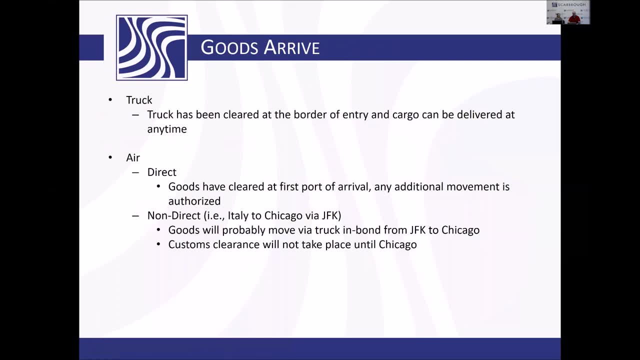 it left and when it's supposed to arrive, But there's not a lot of additional updated information that you're going to see until it actually arrives in the US port in the United States- New York, Seattle, LA, whatever it might be. So when the goods finally do arrive, let's talk for a 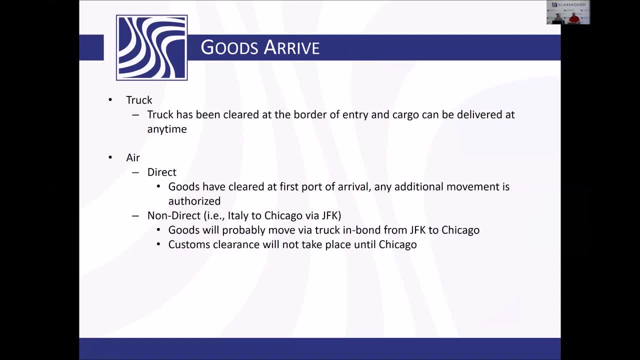 second, real quick: what happens when goods arrive in the United States? First let's look at truck, a truck shipment clearing the Mexico and or Canada border. That truck, the moment that it crosses customs, entries will have been filed and so forth. it will clear customs. That's where it clears. 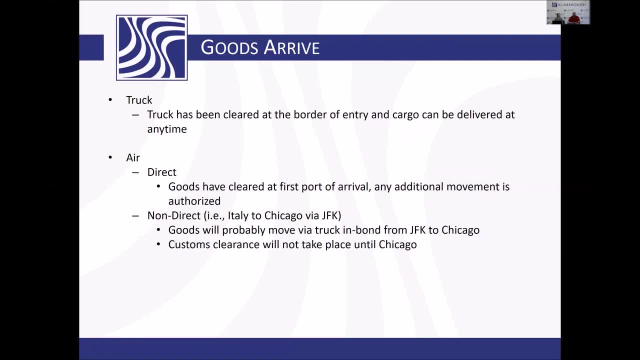 it clears at the ports. clears at the ports, typically right when it crosses, which is good. Air freight, air freight. we see air freight Chicago directing to, or say, Shanghai directing to Chicago or Italy directing to Chicago. whatever it might be, typically customs clearance will happen there, unless it's some. 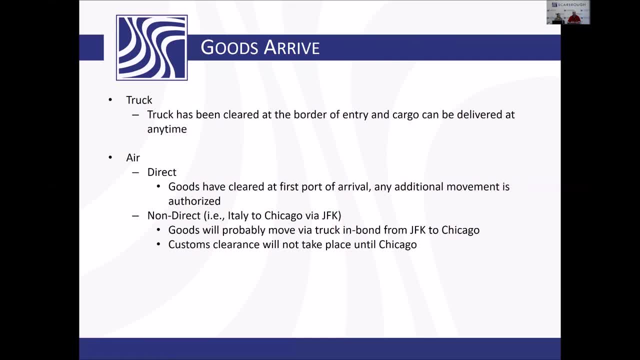 already got an inland destination point, For example Kansas City, where I am today. most goods that fly in they will fly into Chicago or Dallas and they'll truck to Kansas City on a non-direct basis and then they'll customs clear here in Kansas City. So anyways that that. 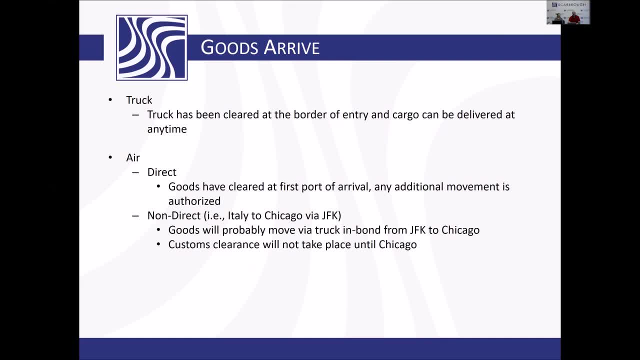 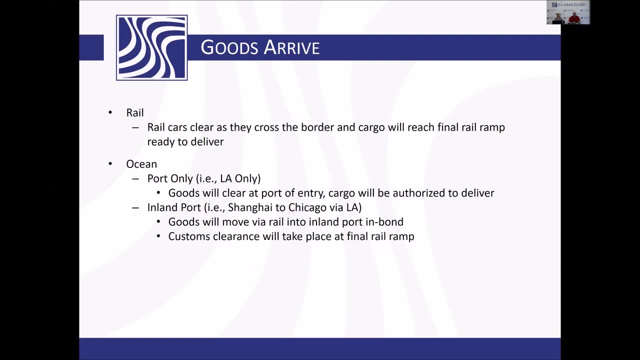 that might change, but it's all based on where the end destination is, typically where you're going to clear customs, and that's a good thing. Rail cars: same thing. rail cars clear at the border as trucks. Oceans- again ocean shipments. we've got a couple variations. there is that an ocean shipment could. 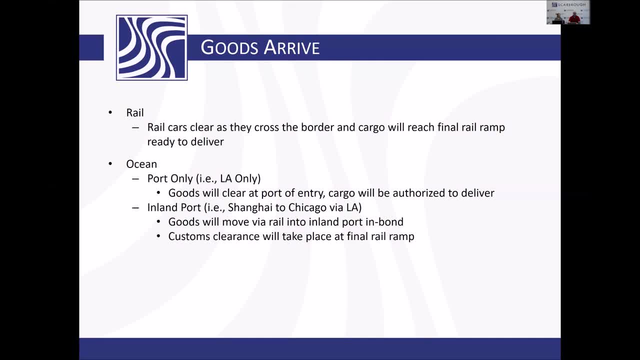 sign to Kansas City, where I am. it could clear customs in LA only, or it could clear customs at the inland port. So it could clear customs in Kansas City. it could clear in Chicago or Des Moines or Omaha, wherever the shipment is destined to. Now what my recommendation is is I recommend that you 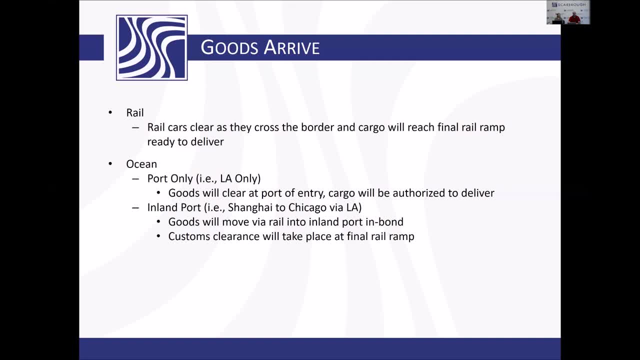 customs clear at the port that's closest to you, so that that can become your home port, so that you as an importer will start to begin getting a relationship with your, with your local customs agents. So, for example, my clients that customs clear in Kansas City, that we have a lot of 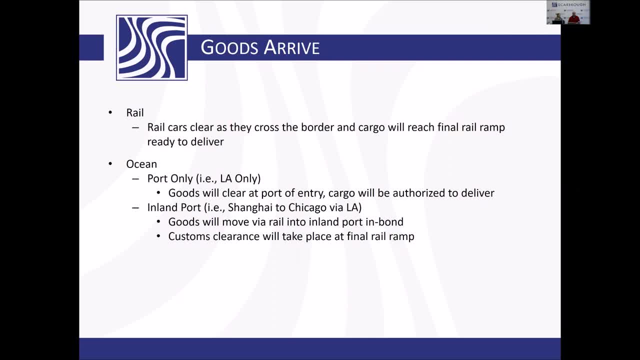 cargo that goes through LA but it moves in from LA and it moves in bond all the way to Kansas City. So that also gives us the opportunity that should there be something wrong- maybe we don't have a document to customs clear the shipment- that we've got a little, some additional more, some. 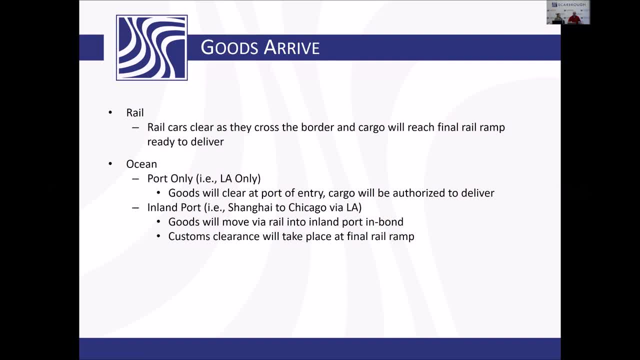 additional time as well to customs clear the product Because I want, I want it to clear here for one. if something goes on an exam, it's cheaper for me to clear to handle those examinations in an inland port. So if it's Kansas City, Des Moines, Omaha, Chicago, Dallas, 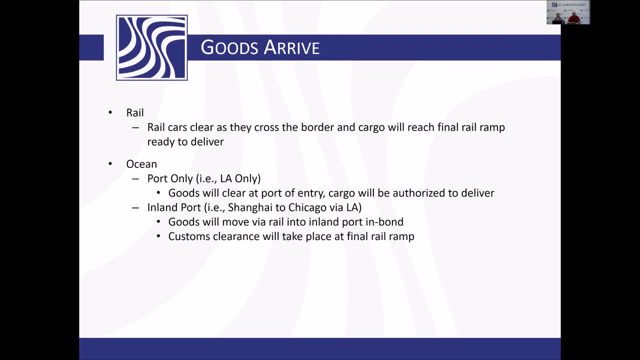 those ports are easier and a little bit more cost effective to handle examinations than, say, New York or LA, because those are some of the largest entry ports in the country. So I recommend that you get a relationship with your customs agent. try to clear it at what we would call your 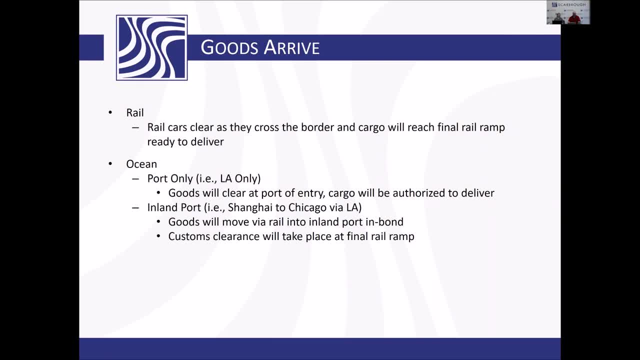 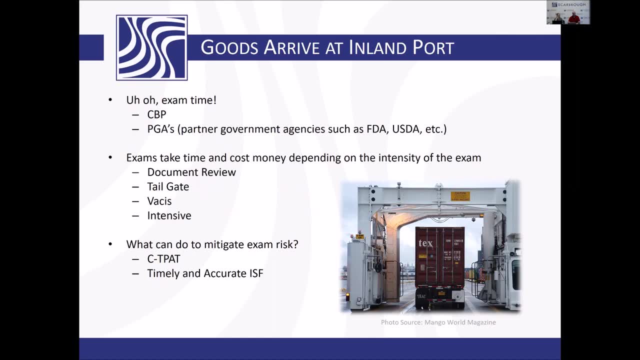 home port. I hope I'm getting through this quick enough so that we have time for questions. So when something, something shows up here, goods arrive at an inland port, things can happen. we can have examinations. We can have from either US Customs and or partner government agencies- We used to call them other. 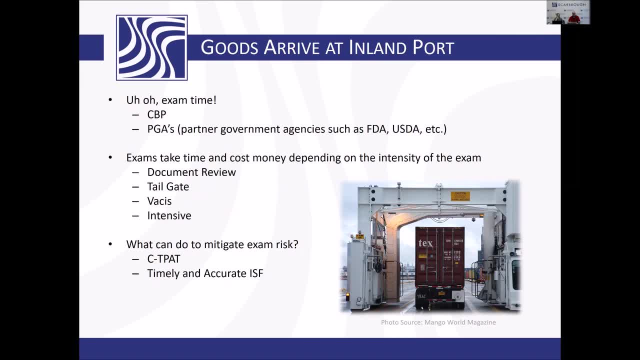 government agencies, But everybody now is is kind of linked into customs A system. so flagging, flagging items for examination and things like that are something that US Customs is doing all the time, And these customs exams, these can be just document review. 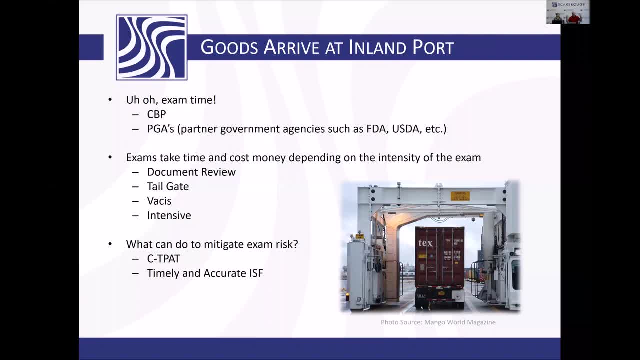 they can be a tailgate exam, where they just go open up the back of a container, make sure everything looks all right. we can be have a BACIS, which is an x-ray exam, or we can have an intensive exam. Now, it's important to note that that exam can happen anywhere in the movement of the goods. 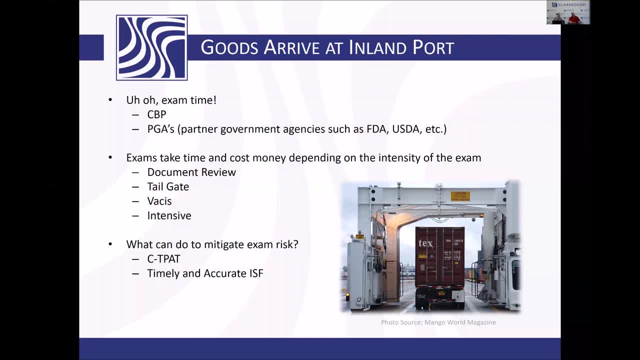 in the United States So that exam can happen in LA. Even if I'm customs clearing in Kansas City or Chicago or Dallas, that exam can happen there. It can also happen in my local port of Kansas City, Chicago, Dallas, Omaha as well St Louis. 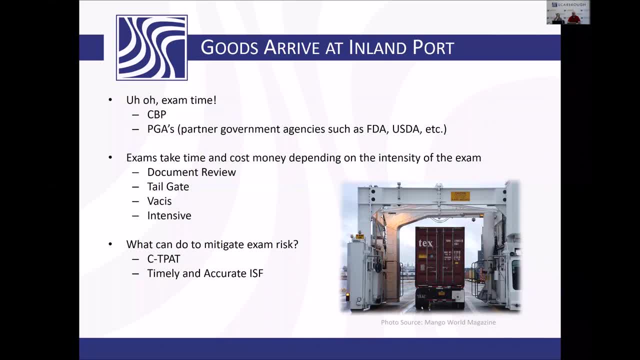 exam can be flagged by customs agents in any one of those ports and it can also be flagged by those partner government agencies like the FDA, the USDA, EPA, etc. okay, because we've got to remember that US Customs is the enforcement arm. they have their own regulations but they also enforce. I believe it's over 400. 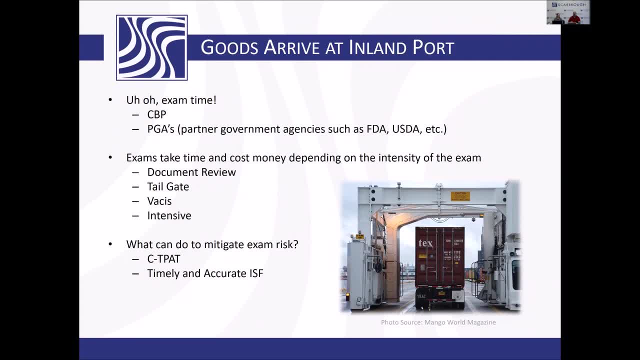 regulations from partner government agencies. so if one of those partner government agencies, such as the USDA or FDA, flag something for exam, then US Customs conducts that exam, usually with with those partner government agencies and reports back. so while I'm why I'm telling you that is because as customs, 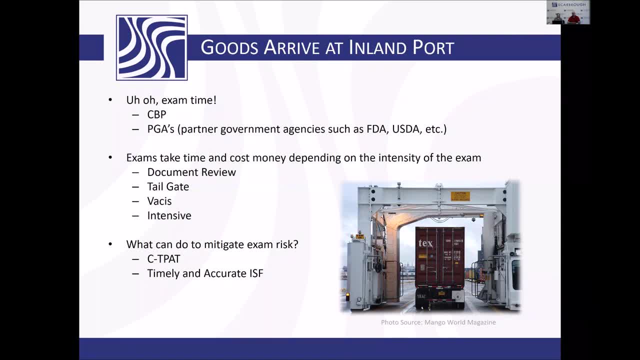 brokers we get access to, to see who actually flags things for exams. so that's information that you'll see on our track and trace programs. that's information that we'll see that, although it was flagged for exam, you know a knowledgeable importer can ask: well, what, what kind of exam? USDA, FDA, or just a US Customs exam- and then 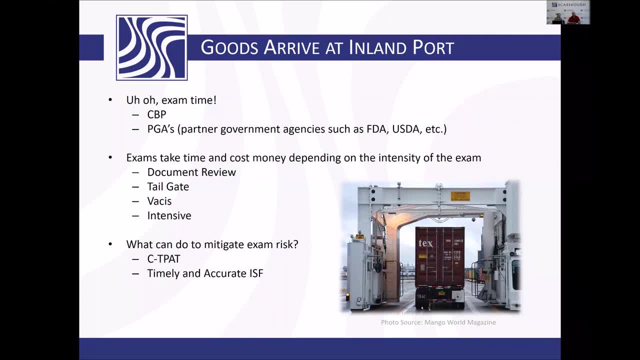 what type is it? a Bacchus, meaning an x-ray, or is it an intensive exam? because, as you can imagine, an x-ray exam is much quicker than an intensive where they're going to unload everything and look inside the box if it's a, if it's an. 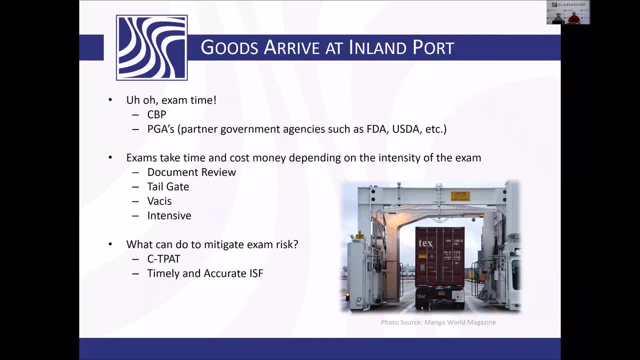 ocean container or air freight, whatever it might be. so those are the different kinds of exams that can happen here at the ports and I'm happy to talk more about that through questions and or one-on-one after this event. things that mitigate exams: ct-pat customs. 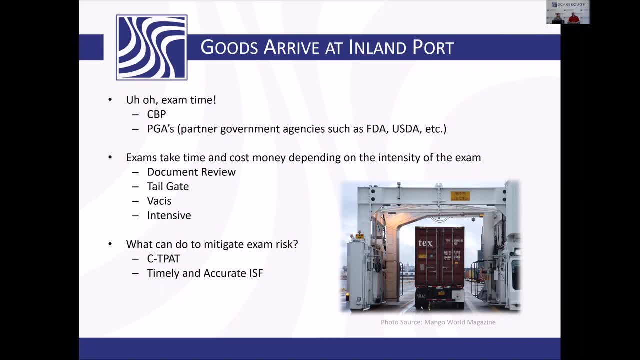 trade partnership against terrorism. that is a voluntary program. many of you that are on this call today are members of CTP at Scarborough is a CTP at consolidator and customs broker as well. timely and accurate is s. if they're timely and accurate, then you don't have to worry about an exam because of them. 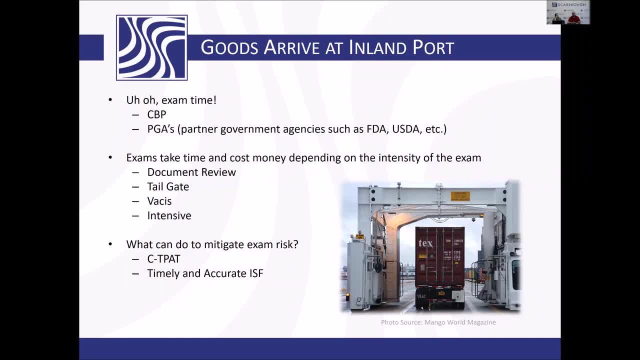 being late and or not not correct. Those are things that help to mitigate the number of exams that are out there. If you're a company that's interested in pursuing CTPAT, let us know. Send me an email- My contact information is on there and we can let you know what that costs to do for. 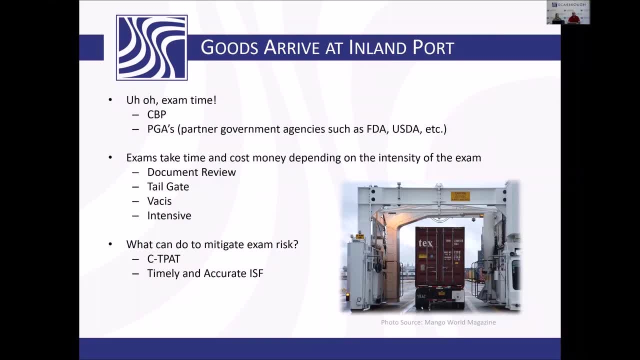 a company like ours to do it and or give you some instructions. if you want to try to do it on your own, That's okay too. But anyways, we're happy to encourage you to also become CTPAT members. At some point there will be some sort of trusted trader program that Customs tries. 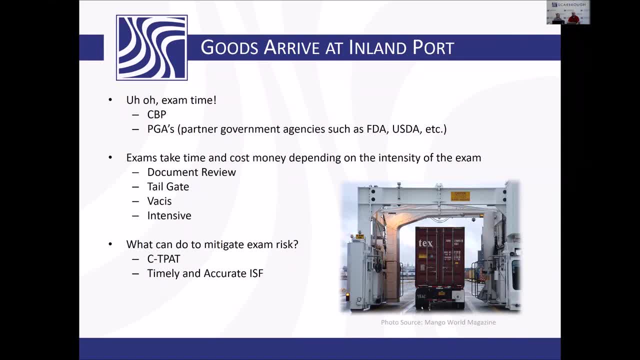 to roll out, I believe, towards the import community. It's the same as getting your TSA pre-check, or like global entry: when we travel overseas and we come back, that Customs knows a little bit more about us and therefore they trust us a little more, and that's really what the CTPAT program is about. 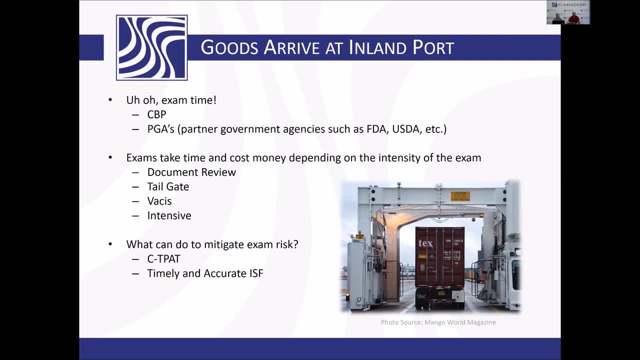 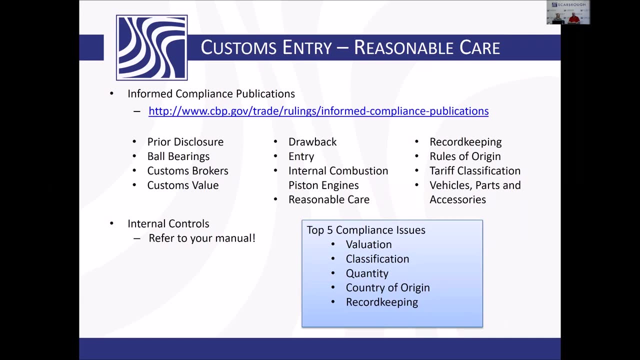 There's importer self-assessment. There's different programs out there. We have broker-known importer programs and we can talk to those. but this is a little more in the weeds than we're trying to do here at the 101 today. So let's talk quickly about the Customs entry process and try to finish up on that as it. 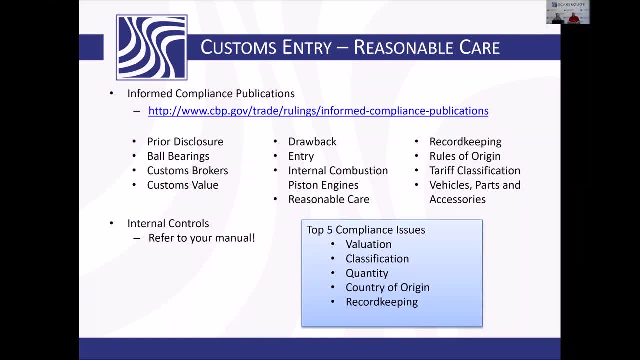 relates to Customs entries and Customs compliance. You, as an importer of record- that's on this call today- you have one standard of care and it's called reasonable care, And reasonable care is usually measured. It's measured against your peer companies, so it would be measuring yourself against. 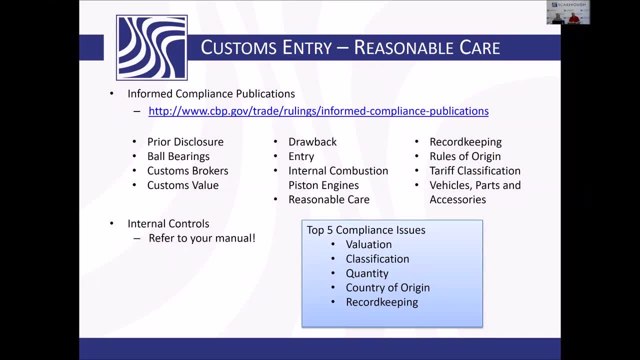 a company of your same size, your same capabilities as someone else. So, for example, a small business that's importing, you know, 52 entries once a week is not going to be measured with a large company that's importing, you know, 100 entries a week, because, 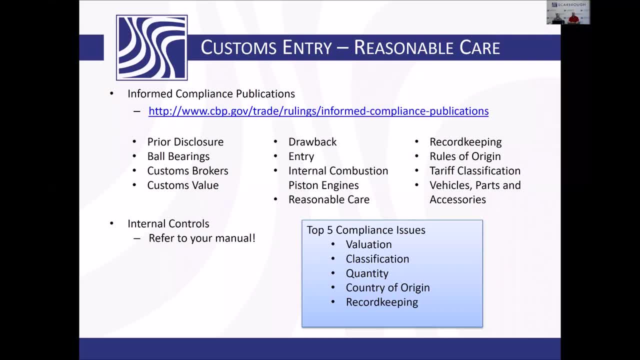 the skill level and the knowledge level would be different, The number of employees would be different, The complexity, The complexity of those imports would probably be different as well. So they're going to measure you based on your peers and that standard is reasonable care. 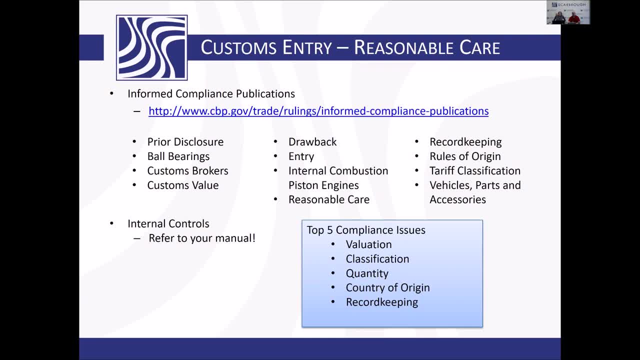 And reasonable care really means that you're going to try to do to the best of your knowledge and ability, the best that you can Now, believe it or not. attending trainings like this one and the ones that Scarborough does on a monthly basis actually is one of those mitigating factors towards your reasonable 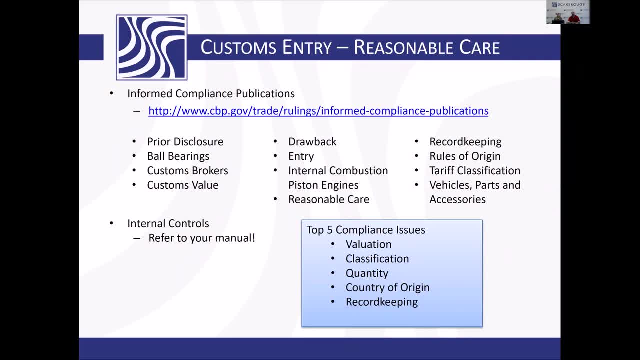 care standard. It means that you're engaging in training from a licensed Customs broker and knowledgeable group As to the laws, regulations and things as it relates to import trade and then taking that information and making sure that you're doing the best that you can. 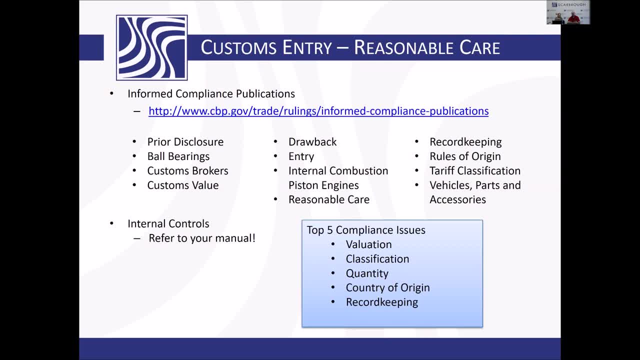 So by attending a webinar today on Import 101, you're actually helping to meet your standard of reasonable care. Now, there's a lot of things out there that also help And, as part of the MODAC, when Customs came up with reasonable care as the importer's 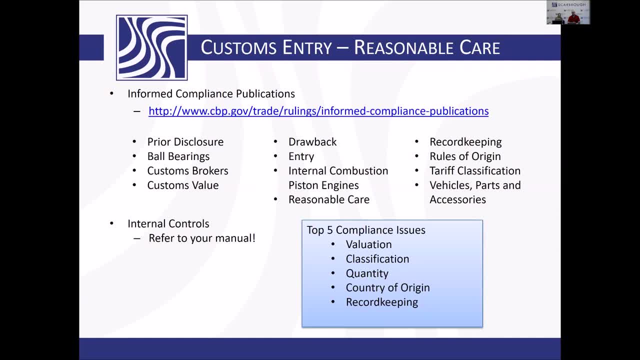 requirement. they also take on a requirement to make sure that you're informed, and they do this through And I've got a link here on the slide and, again, we're going to send these slides out to everybody, along with the copy of this presentation. when it's not, 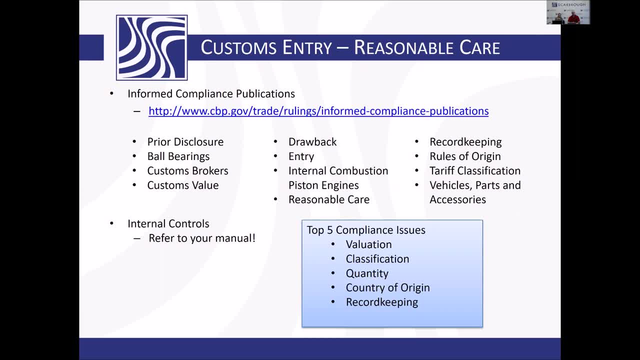 But these slides have. If you go to this Compliance Publications and you read through this, it's got really what Customs is looking for as it relates to these specific things. Now, when we put down here the top five compliance issues are: valuation, classification, quantity. 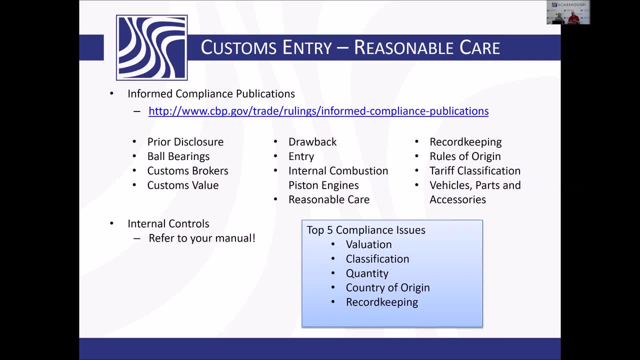 country of origin and record keeping. So I would certainly recommend that you look at the Compliance Publications as it relates to those five topics and make sure that your processes and procedures are in line with those, And we're going to talk about four of those today, just to kind of give you a little more. 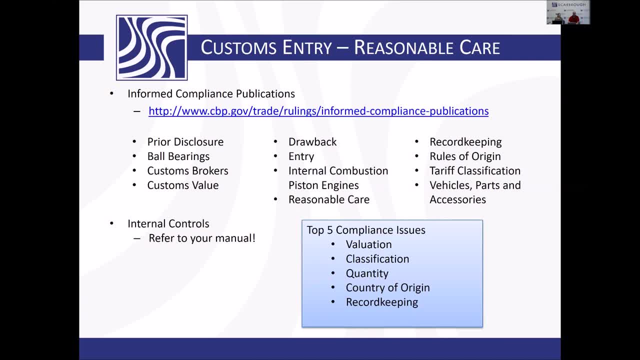 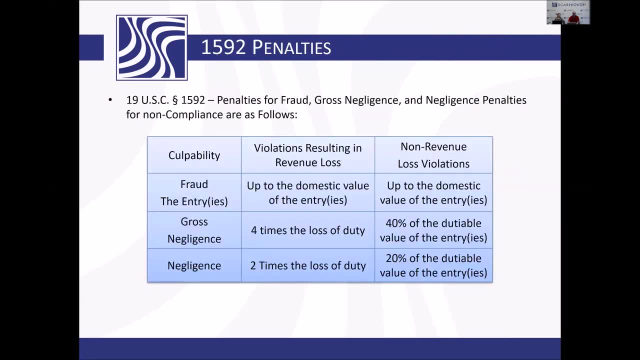 insight into what those import requirements are from a Customs standpoint to meet your reasonable care need. And why do we do it? And the reason is right here. This is why we try to meet your standard of reasonable care. We try to meet the reasonable care standard. 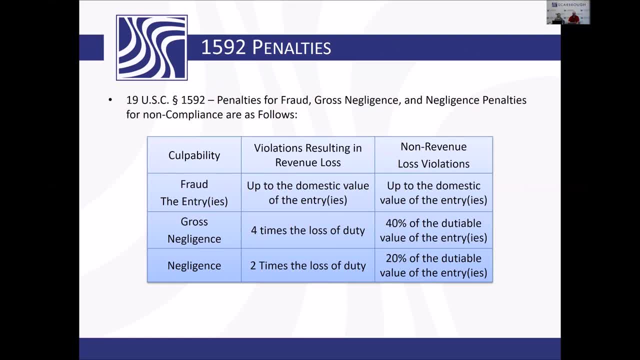 It has to do with penalties, Penalties and the differing degrees of culpability. So the degrees of culpability are negligence, gross negligence or fraud, And here are the related penalties, as you can see on this slide, whether it's revenue. 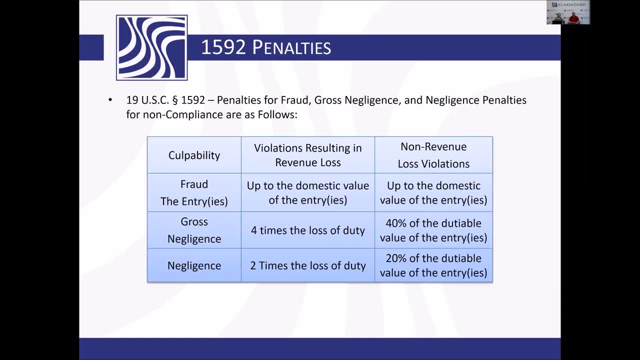 loss or non-revenue loss, what the potential penalties are for doing something wrong, for not meeting your reasonable care standards. If we can meet those, that's great. We still might have to pay additional duties and or some mitigated penalties of some sort that might not be held to these. 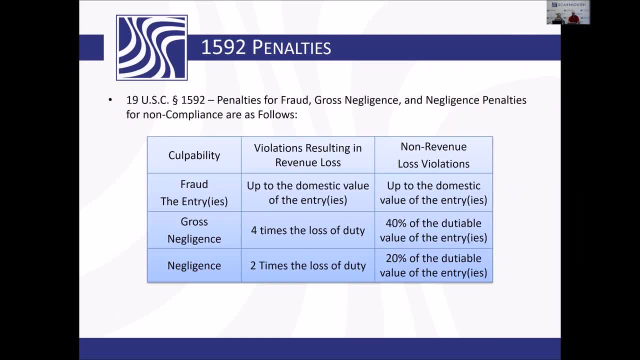 other higher degrees of culpability And, honestly, Scarborough's got a very good client base that takes this very seriously, because we're so compliance driven that I think our clients appreciate that and help us to meet those needs. So let's talk about first entry documents. 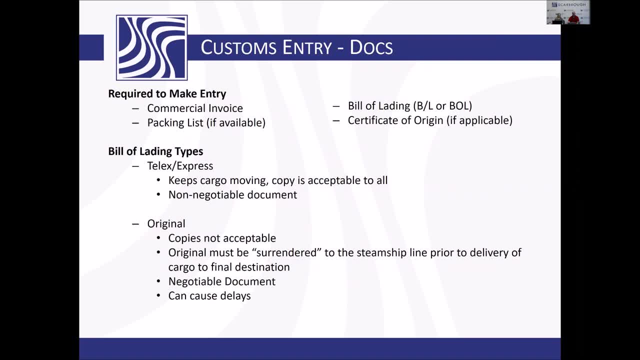 We mentioned them earlier. Commercial documents: Commercial invoice, packing list, bill of lading, certificate of origin. Again, the certificate of origin is really that burden of proof document as it relates to goods. So if it's a NAFTA related, you're going to get a NAFTA certificate of origin. that's going to be. 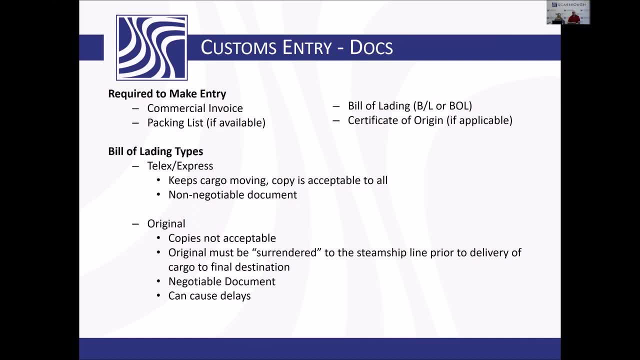 required and or any special trade agreements. virtually all require a certificate of origin, some sort of burden of proof, and or manufacturers have to validate the origin of the goods. We talked about the bill of lading types, And what's really important is that you have to have a certificate of origin. 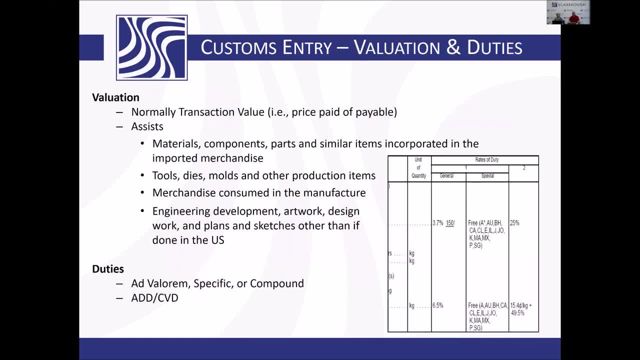 It's required there already, So I'm going to kind of move through that quickly. So let's talk quickly about valuation. OK, There are. there are five methods of valuation. The most common is transaction value And that's what we've got listed here on the screen. 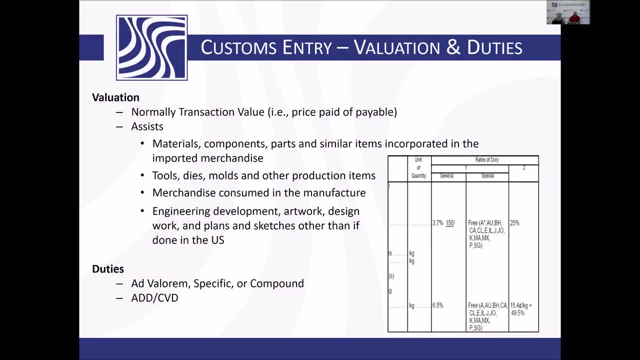 And transaction value is really an arm's length price- paid or payable- plus certain statutory additions. OK, Some of the statutory additions are assists, And now one of those is listed here And assist is a material. OK, So that's what we've got listed here. 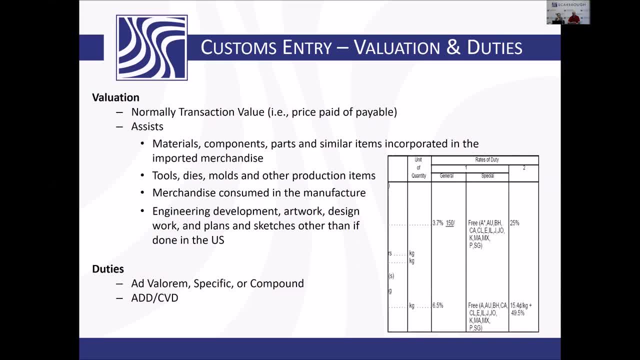 So it's a material component, a part, something that is paid for by you, the shipper, or you, the buyer, you the consignee to usually a manufacturer or someone overseas to supply goods or materials for your product. 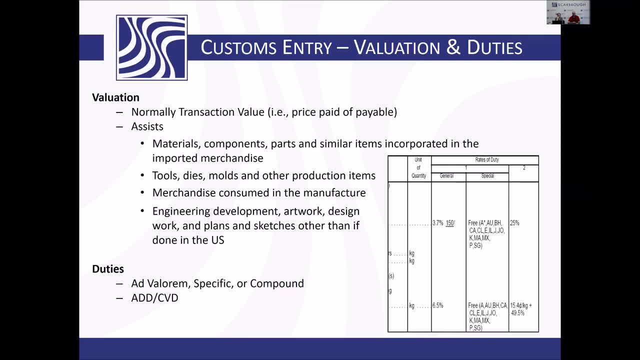 Typically when I'm doing this training out of an importer's location. we'll go in more in-depth into all of the different statutory additions And I can sum them up for you real quick through an acronym. It's called CEA, C-R-A-P-P- CRAP. 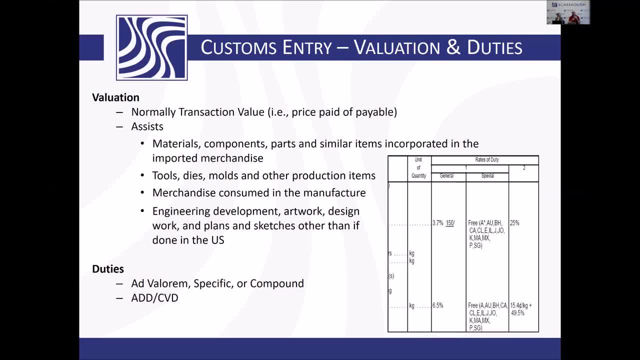 It's commissions. royalties, assists, packing and proceeds. Those are the five statutory requirements that you need to look for, But assist is the number one. So an example of an assist is that, say, I wanted to buy this plastic case for this phone here. 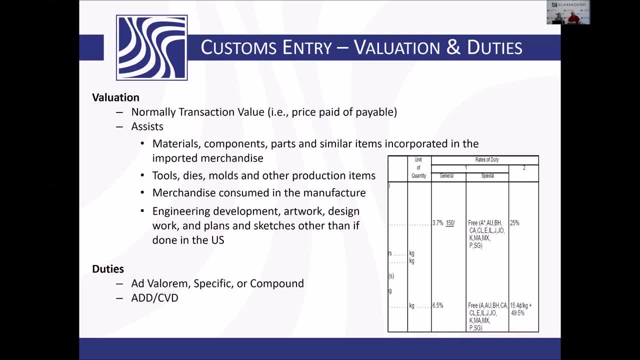 OK, I was going to buy it from someone overseas, But in order to buy this plastic phone case for my cell phone, here I'm going to tab And I'm going to say, hey, I'm going to pay you $50,000 in tooling. 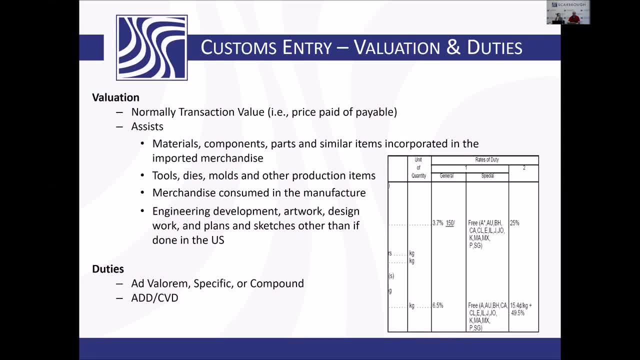 So I had to give him $50,000 up front so that he could create the tooling to make this case. OK, Typically I paid that. I might have paid that six or eight months in advance before I ever see a case. 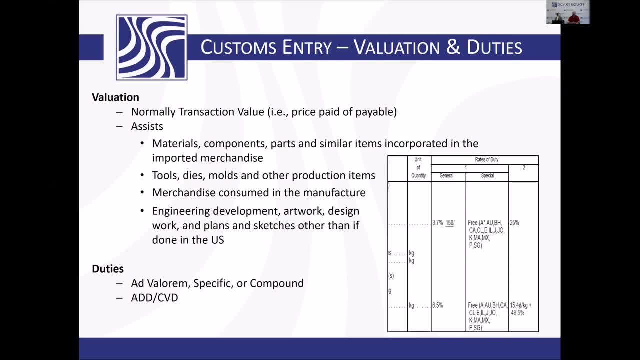 OK, So I paid that $50,000 up front And then my manufacturer starts manufacturing my cases. So when he does that and he's loading, he's creating that commercial invoice. Well, now that commercial invoice, He's only going to charge me for the cost of making that good. 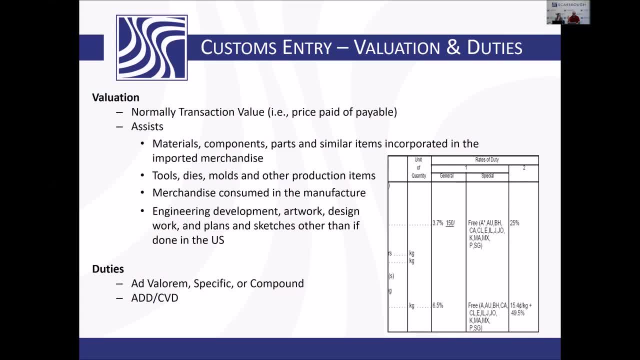 So his labor and plastic prices and things like that. So maybe it's only a dollar to build that case that I just showed you. OK, So it's a dollar for the case. Well, the fact of the matter is is that I've already paid that $50,000 for that tooling. 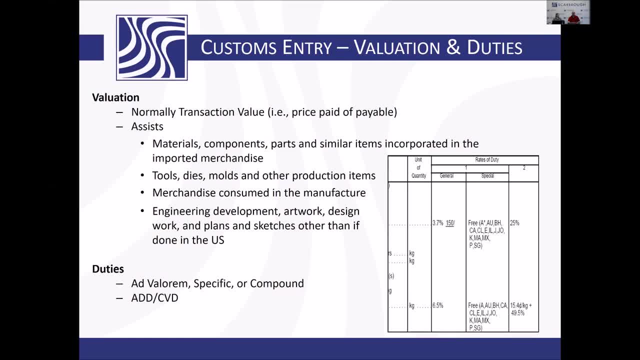 I need to also include that $50,000 on the cost of my import, Because my cost of goods is not just $1. It's actually $1 plus the cost of tooling. So you can see how an ASSIST could sometimes get missed and not be included on your invoice. 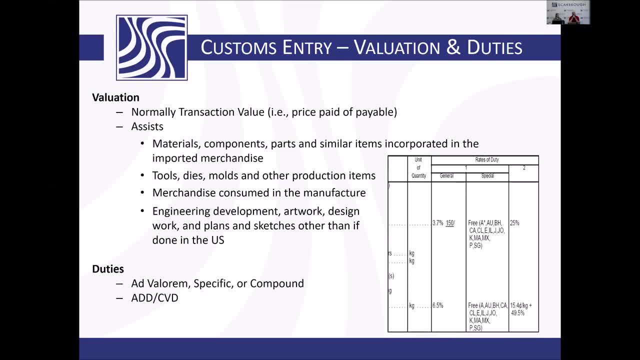 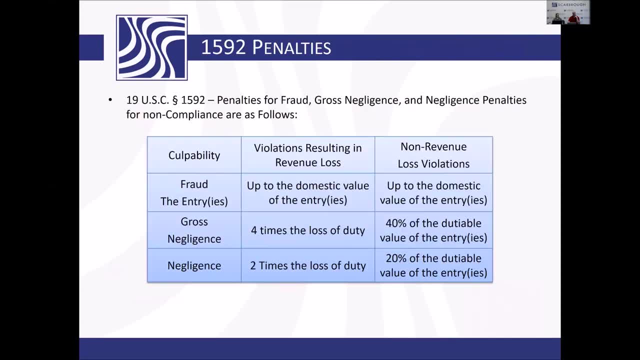 And if it's not included on your invoice, then you're undervaluing your product And thus you're looking at a potential violation, as I go back up here to these 1592s, because you've undervalued your product. 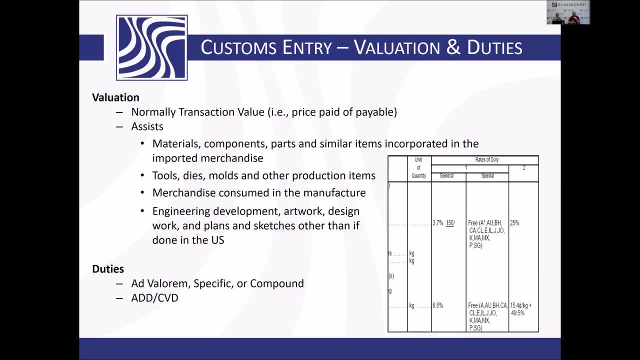 And therefore you've not paid an adequate amount of duties. So those types of situations can happen within your product If you have any of these ASSISTS. they can happen with royalties, commissions, proceeds and packing as well, And we need to make sure that that information gets communicated to the customs broker so that we can handle that appropriately. 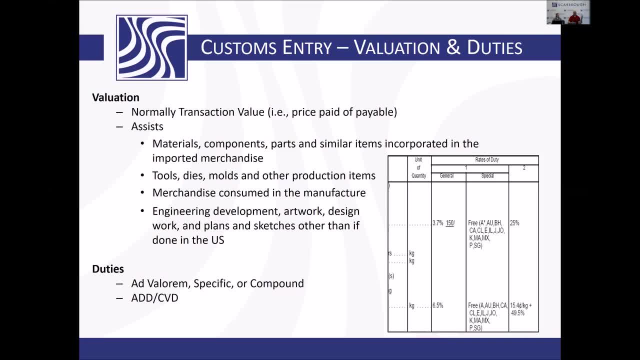 So if you're buying any molds, you're buying any diagrams, anything like that- from overseas and having them sent to your manufacturer. that's a potential risk there. So we would like to talk to you about that. Give us a call, We can help straighten you out and get you back on track. 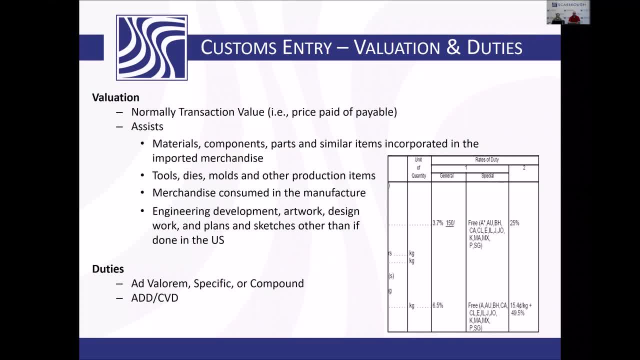 We can get you back on the right path. if that's there And what that does is determining the value of the product correctly, really helps you determine what the total amount of duties, Because duties are typically on percentage of value. There are some that are compound duty rates and are rated based on the amount of product that you're bringing in. 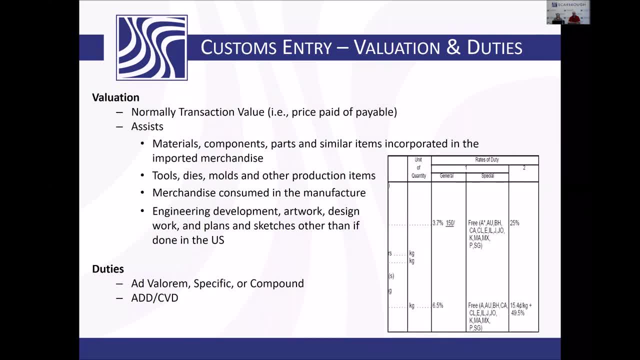 But I've got an example here of, say, 3.7%, which is close to the average duty rate out there. I have a question that just popped through Yep. This person is asking: what about commissions paid on the US side? 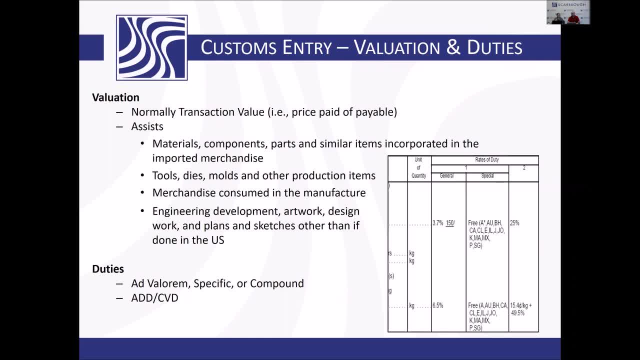 Should they be added to the import value as well? That's a good question, and it's one that we're probably going to have to have a little more info, because there's usually two types of commissions. There's a seller's commission, the commissions from the seller overseas. 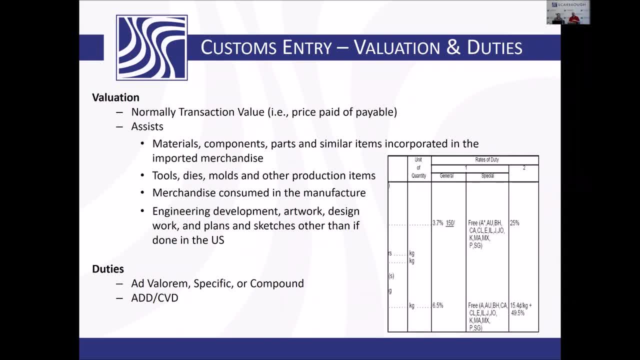 And then there's a buyer's commission here in the US and we probably need to get the details more specific to your situation. But if it's your person here selling a good and making a commission off of it, that's probably irrelevant because it's after the importation has been purchased. 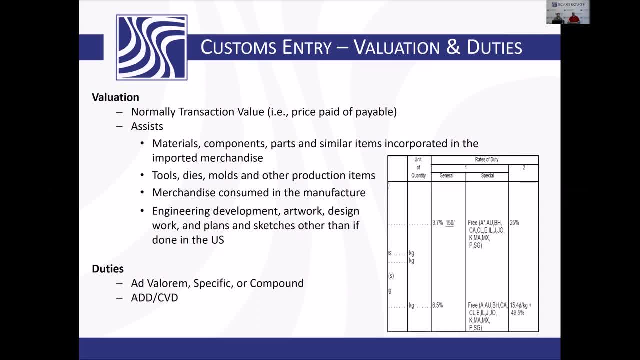 But it's typically an agreement. a commission is typically an agreement that is between the seller overseas and the buyer. here And again I have to get into the nitty-gritty of the actual contract per commission That would pay him and say your vendor overseas, the supplier overseas, some sort of commission. 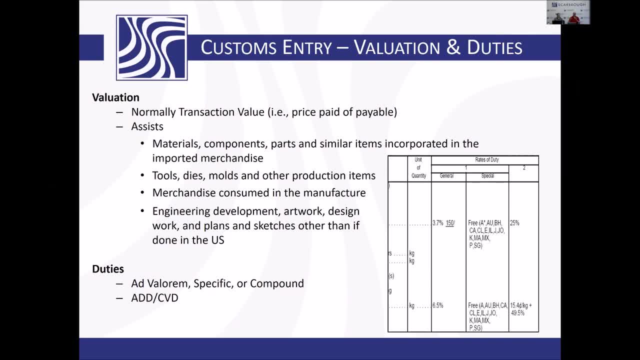 Based on the sale of goods here in the United States. that's usually the type- And some can relate that to royalties as well- based on the number of sold. So I'd have to look at your specific agreements And if you want, after this event, to engage us in that conversation, we'd be happy to help you with that. 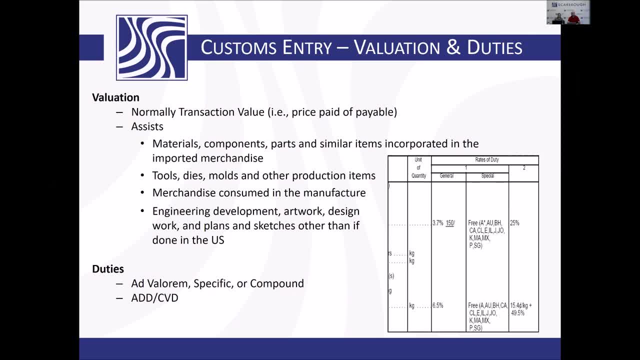 Yeah, definitely send us over an email, because we don't know who submitted that question. I've got one more question here, Kevin. Can you repeat the CRAAP acronym? Can you repeat what everything in it stood for? Yes, yes. 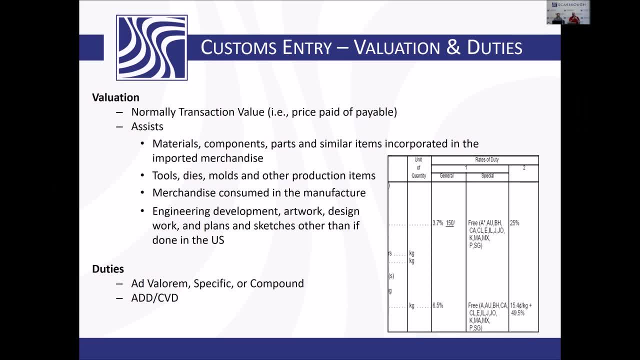 Commissions, royalties, assists, packing and proceeds. Proceeds would be subsequent to sell of a product. Again, that's money going back overseas to the vendor that would need to be declared. So, anyways, that's what the acronym stands for. 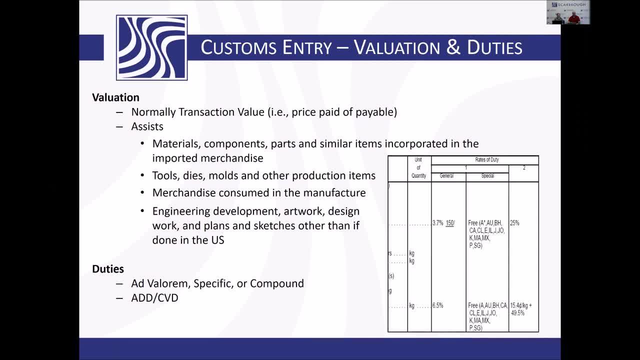 And those are typically the other statutory additions. And I love acronyms because that one will stick with me the rest of my career. It has, since I've been doing this for 20 years And it's one of my favorite acronyms. 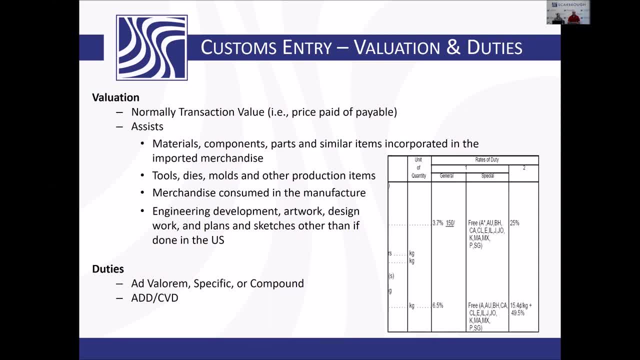 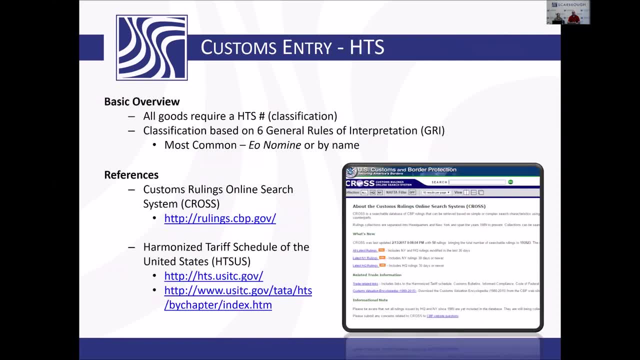 It's one of my favorite ones to use because it is It's price paid or payable and all that other crap. So let's move on to HTS- classification of products- And again, this is a one-on-one course, So I could spend- honestly, I could spend- a half day of training for valuation tariff classification. 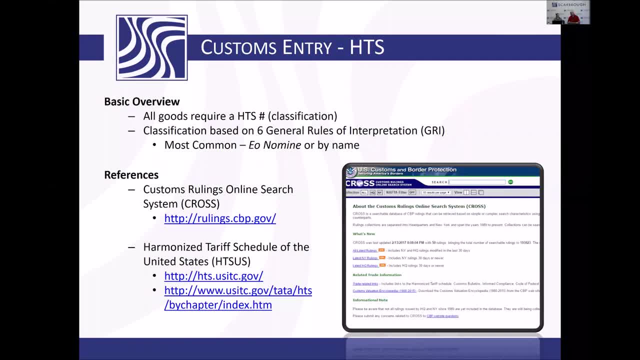 record keeping and country of origin markings, And we're trying to do it here real quickly And we need to move a little bit faster to get to all your questions. I know, Yeah, about 20 minutes, All right, So, HTS, the basics for this is that all goods that are imported require a harmonized tariff. 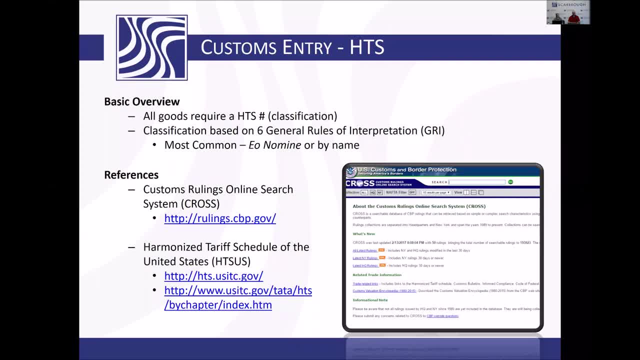 system number. The harmonized tariff system is universal to a six-digit level in the 196 countries that subscribe to the harmonized tariff system. OK, In the United States we add four additional ones that are really more specific for census purposes. So we've got a 10-digit harmonized tariff system number. 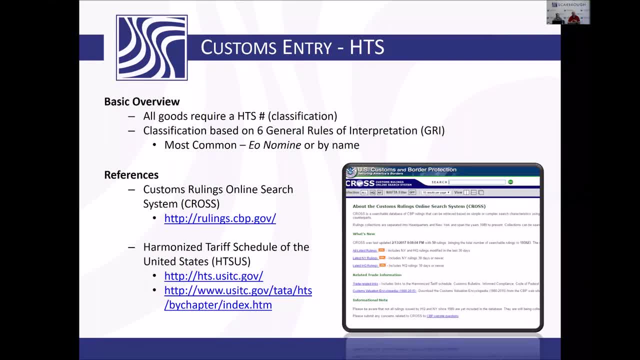 And typically that information is the same. It's based on what is the product and how is it used, what materials is it made out of, and things like that, And those are all the questions that we ask you every time, because many of you were engaged. 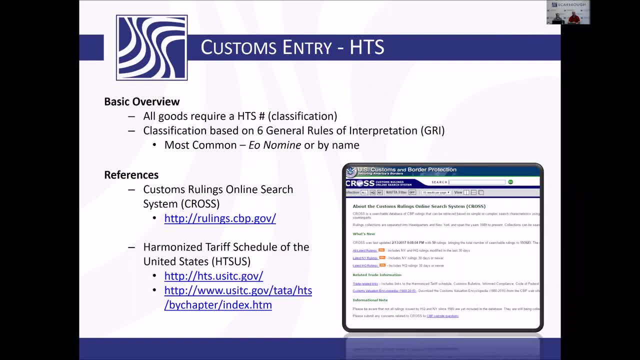 in product development: looking at products before you're looking to source them, in order to determine what the duty rates will be and if there's any other obligations, such as anti-dumping duties or countervailing duties and so forth. There are some tools that's out there, and I've included one here on your screen today. 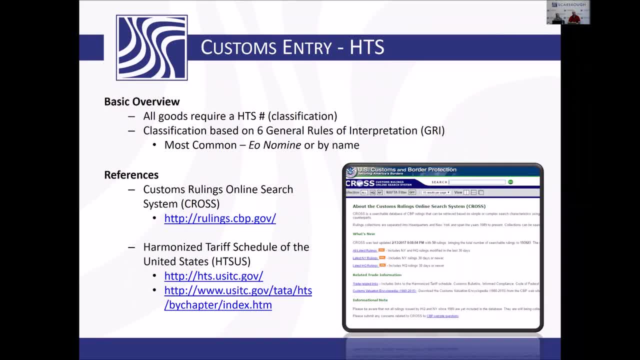 And that is the Customs Ruling. Online Search System- Acronym is CROSS. If you go there, you can input some of the characteristics of your product, what your product name is and some additional info and it'll bring up where Customs has done. 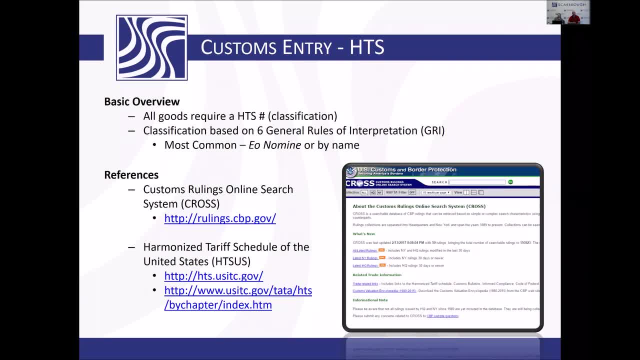 some rulings, maybe on similar products, to help you identify what the harmonized tariff number is and what the applicable duty rate is for that item as well. So, anyways, it's a great tool. This has been developed in my lifetime. We didn't have this when I started doing it, but it's become a great tool. 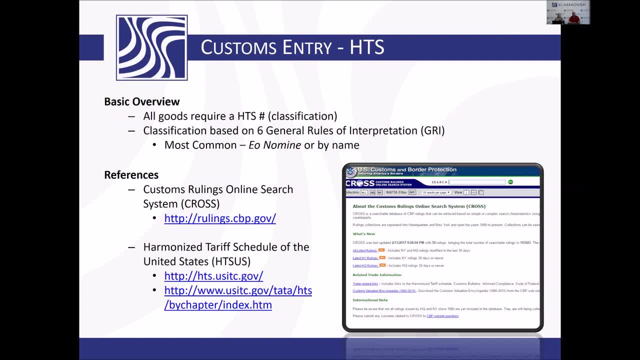 It's a great tool for folks to look through rulings and see what Customs is thinking as it relates to specific products. The only thing is that this is mainly on products that have already been imported. What if you're doing something that's brand new? 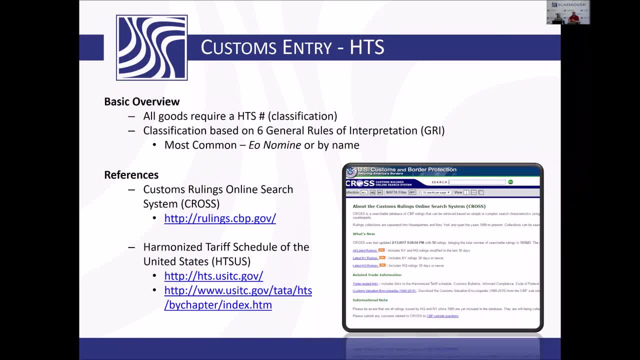 Then what you're looking for is: you're looking for something similar to kind of point you in the right direction of the harmonized tariff system, and what number of years would be. So I've got a link here to the harmonized tariff system as well. 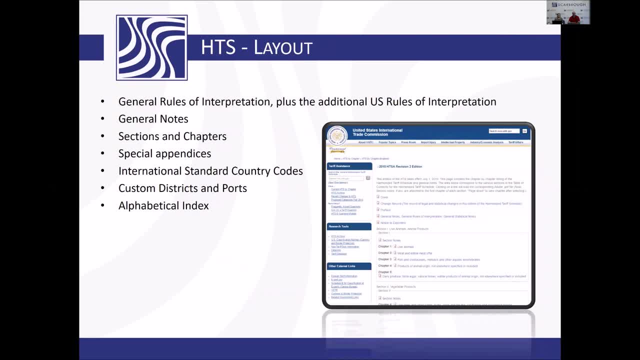 There's really a list. Okay, There's a list of rules that we're required to follow when we go through the classification process And unfortunately, one of those is not looking at cross We? as a Customs broker- myself as a Customs broker- I follow the general rules of interpretation. 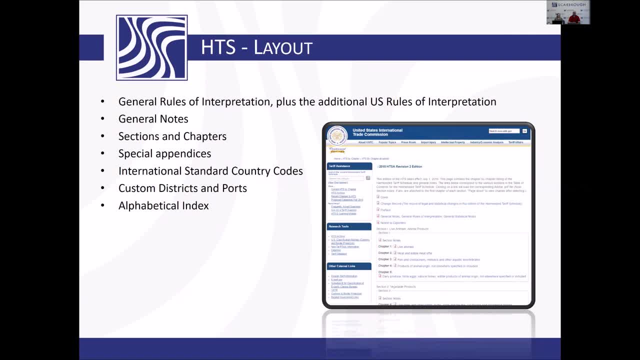 I look at the notes of the chapters, the sections, special appendixes and things like that in the harmonized tariff system itself to come up with that answer. And then typically I utilize cross to cross-reference my answer to make sure it's right. 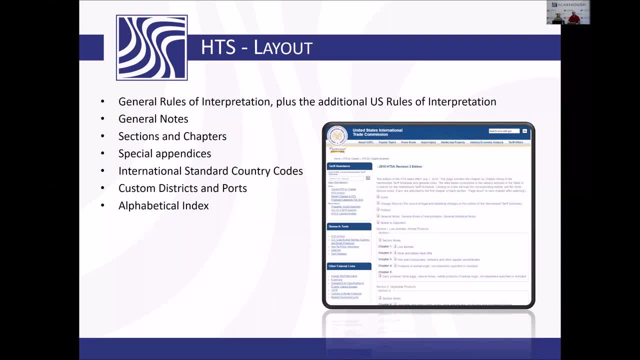 But, anyways, there is a specific format for doing it And that's something that we teach in really a half-day course on how to properly classify your goods. It's something that we give to people that are in research and development: R&D those. 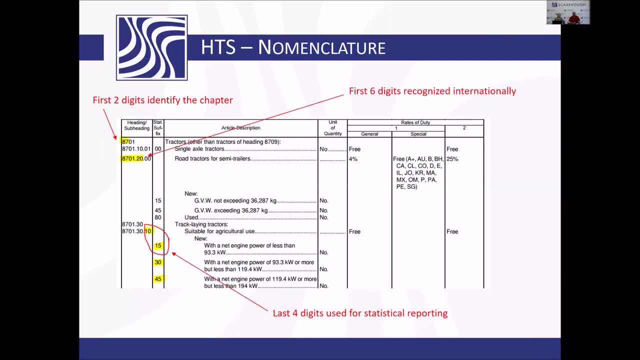 kinds of things. And this is what it looks like for, say, a tracker here Is that you've got the first two digits, which are the chapter, you've got the next four, which is the heading, and then you've got the subheading and then you've got the last. 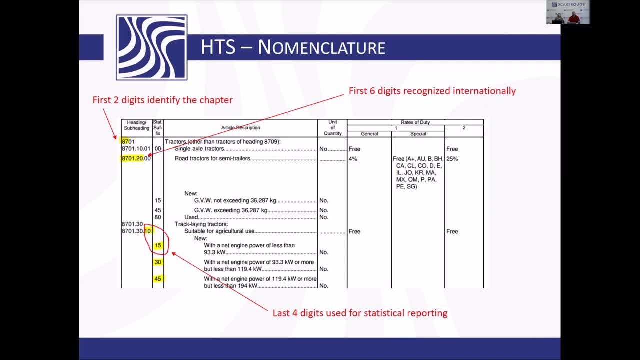 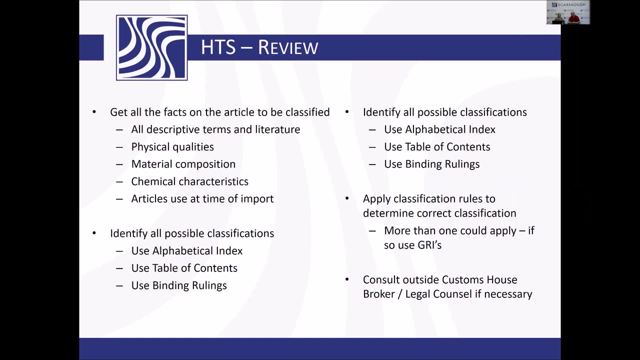 four numbers for statistical. It's just for reporting purposes. So anyways, that's in here for you to look at. Can I ask something real quick? Yep, Because this came up the other day: Do HTS classifications expire? Let's say, for example, an importer says: well, this is just what we've been clearing. 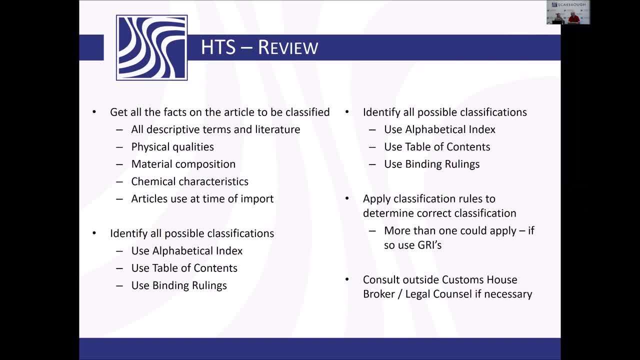 this under for the past 10 years? Is that something that they should look at and review? I would encourage people to look at their tariff numbers On an annual basis. typically, the harmonized tariff system will make a couple of changes a year and they'll issue those in supplements to the tariff. 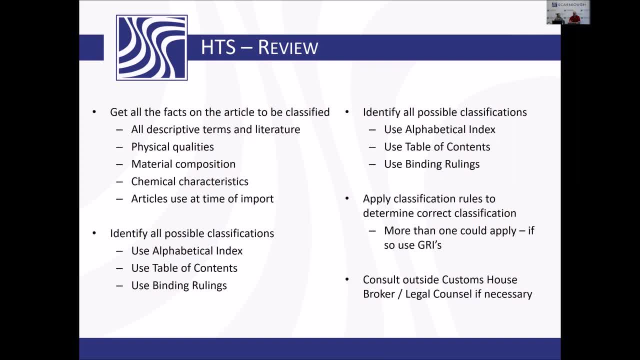 And it might change the last couple of digits for reporting purposes, and or it might not change, But there are times that certain things expire And, specifically, as the miscellaneous trade bill that's usually passed through, Congress has usually some provisions for some Chapter 99 tariffs and those Chapter 99s usually. 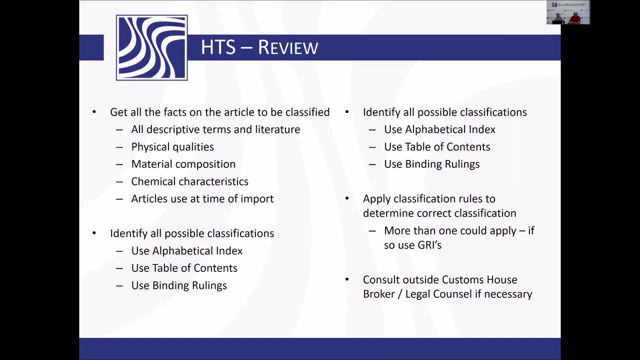 provide maybe some duty-free treatment for some goods. It's over a certain period of time, And when that miscellaneous trade bill expires, so do those tariff rates. For example, I remember doing a big project on batteries years ago and it was part of. 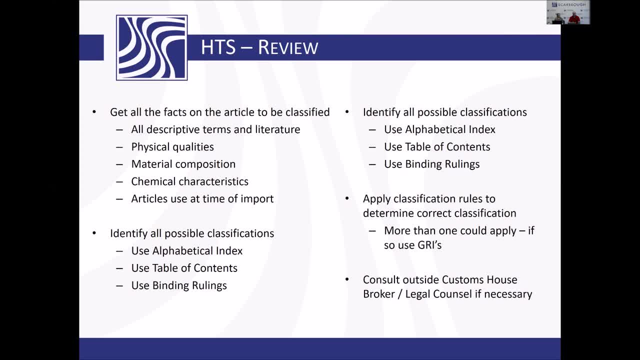 the miscellaneous trade bill And then it was only valid for certain dates, But anyways, during those dates they got to bring in goods at elo-produced duty and or free duty using a Chapter 99 tariff number which was included in that miscellaneous trade. 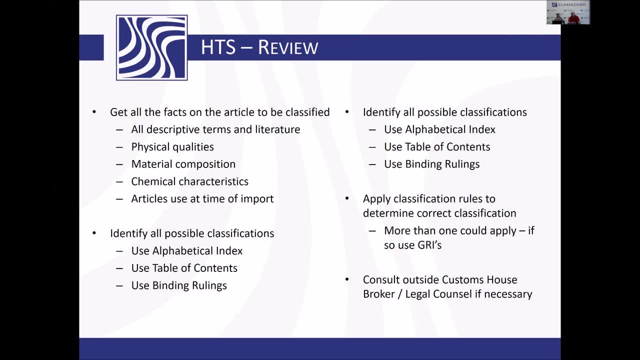 bill, So that's something that gets a lot of heat in our legislators, But anyways, it's possible. I would re-look at it every year just to make sure it's the right one. So to ensure that we're staying compliant as an importer, we need to review our HTS. 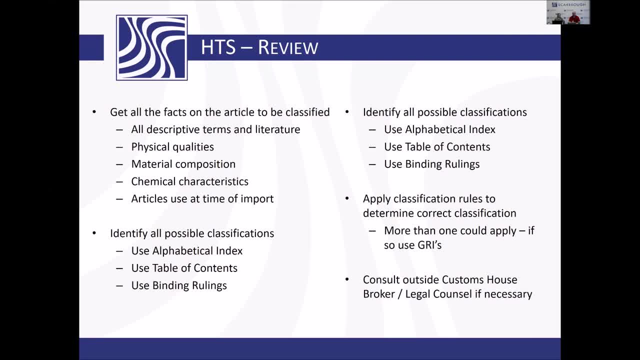 classification and HTS numbers we are using. Yes, Absolutely. Thank you. So again, here's kind of a review. These are the things that we, as a customs broker, ask: description of terms, physical qualities, materials, composition. You know this is great. 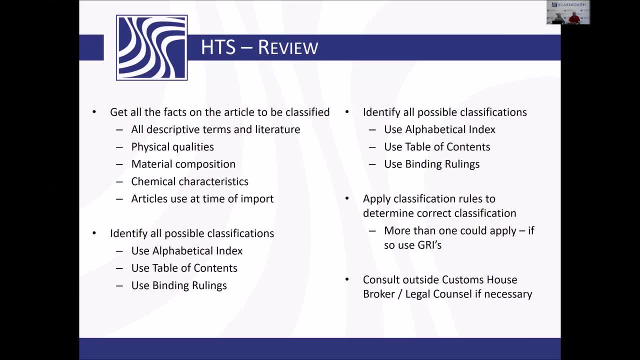 This is great because you know, the adage here of garbage in, garbage out applies all the time. I'll give you one example real quick: a seal. If I said, okay, I'm importing seals, Kim, What would you think of? 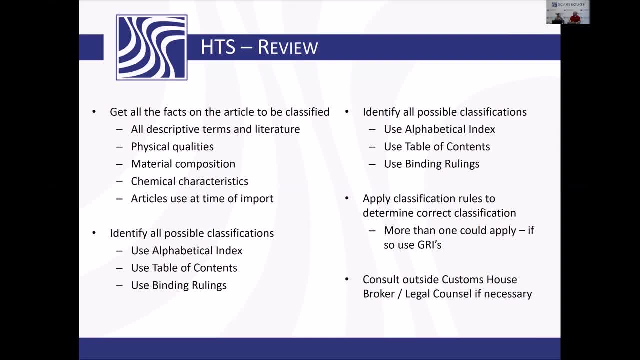 You're importing seals. Yeah, Would you think I'm bringing in a live animal and not live animal or a rubber seal or a plastic seal that goes in as a component, part of manufacturing. Again, that's a great example, because you've either got a live animal or you've got a plastic. 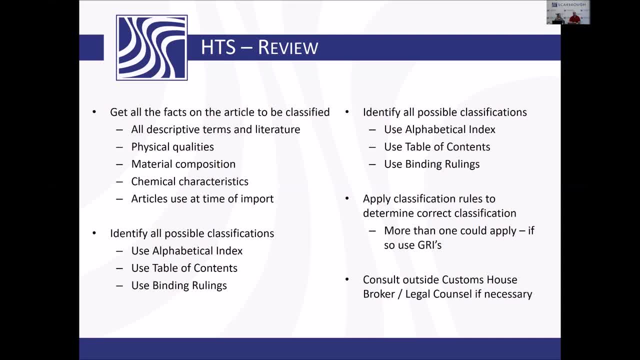 or a rubber part for the most part. So you've got to have really good descriptive information when you're importing. That information should be in your ERPs and it should be on your purchase orders and it should be on your commercial invoices, because if not, that's all something that could actually 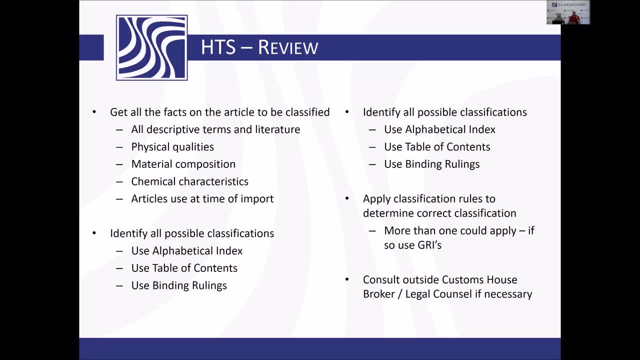 flag a customs inspector for an examination. It is by looking at your documents and then not bringing details. Your invoices just have numbers on them, like your item number, your SKU, without descriptions. That's not really good for customs either. So our idea is: let's give as much information, as detailed as possible, so that we can prevent 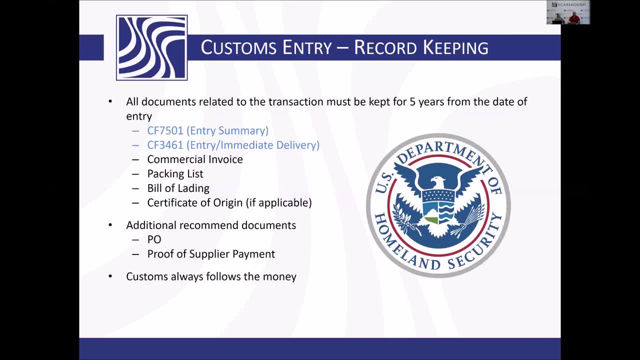 any examinations. Record keeping real quick. Record keeping requirement is five years right now from the date of entry or the last date of activity for your shipment. So if it's anti-dumping or countervailing it might be longer than that, but typically 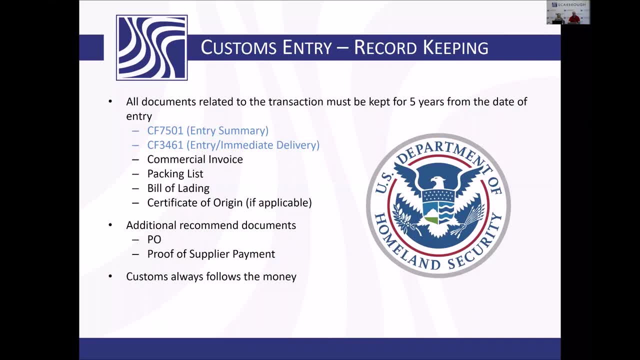 it's five years. I would keep my records and that's all records, from the issuance of purchase order through the payment of goods. So make sure that you have multiple departments involved in your record keeping process. So that's accounting, that's receiving. we want to know exactly the correct quantity. 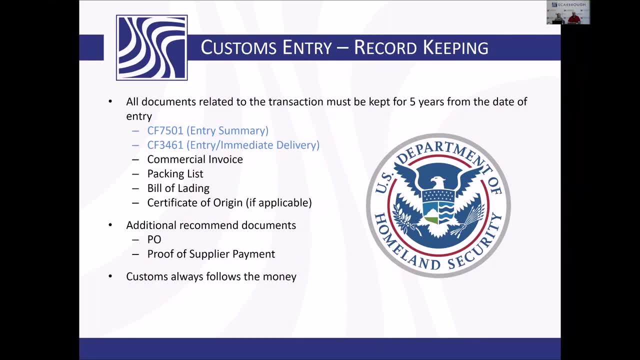 that's received All of those, that those get saved somewhere in a manner that you can recall them if customs asks you. for five years Now we as customs brokers we image all of your documents and you can log in and you can have access to those, but we don't have your payment records. 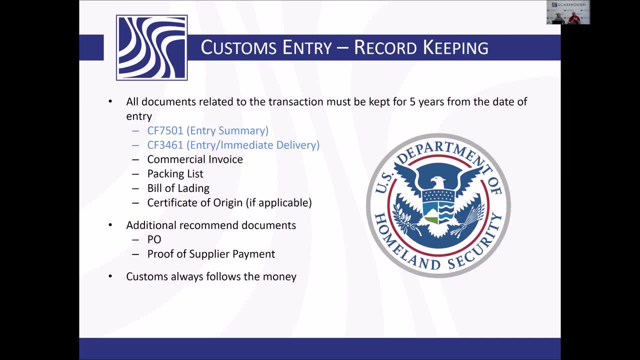 We don't have your receiving reports, those kinds of things that you also need to make sure that you maintain for a five year period to validate exactly what was coming in, And then we recommend at the end of that five year period that you destroy those. 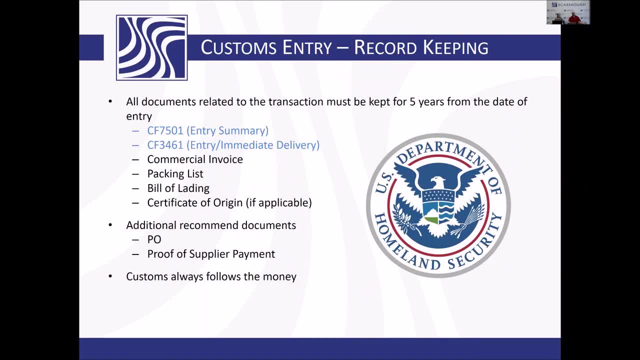 Because if customs comes in to do an audit of your company and you've got seven years of records, they're going to get access to seven years of records. Let's just stick to the statutory requirement of five years. Okay, So that includes even copies of the power of attorney that you've issued to me or the 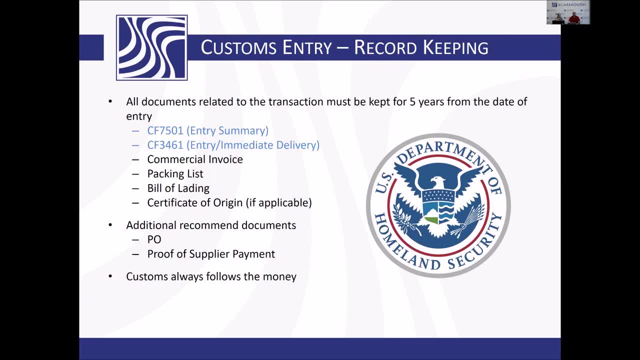 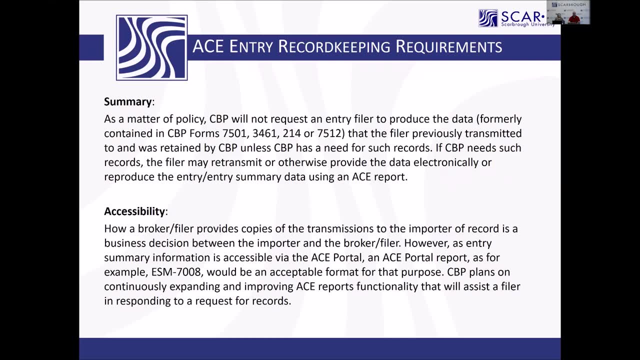 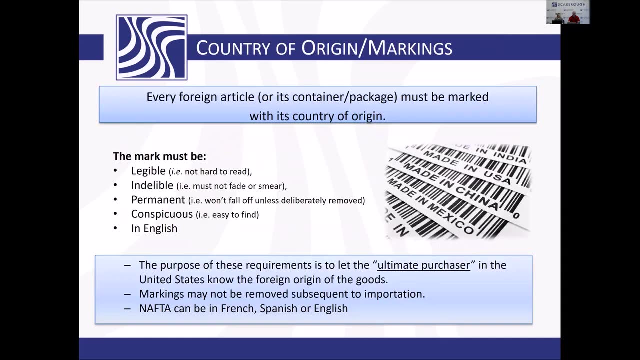 customs broker you're using. There is a slight change with ACE record keeping and meaning that ACE is going to be the main portal of record for maintaining all the documents and some of the documents or the forms that we're accustomed to in the past, such as the 3461 and 7501, that are listed on this page. 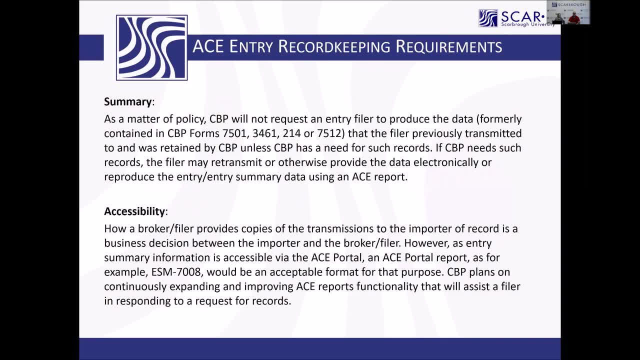 Some of those forms. they're actually going away with ACE and their record keeping Okay, So just want to make sure you're up to date with that. Can you quickly touch on the difference between the 3461 and the 7501?? 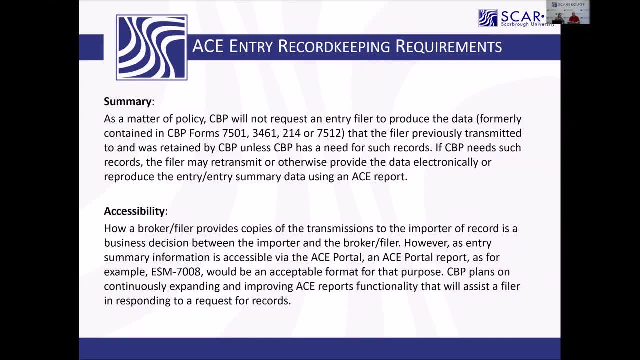 Sure, The 3461 is what's called the immediate release document, And what that means is that that's what you've got to have: to have the initial customs clearance. Okay, That's your 3461.. A broker like us, we transmit both documents, both forms, at the same time to customs. but 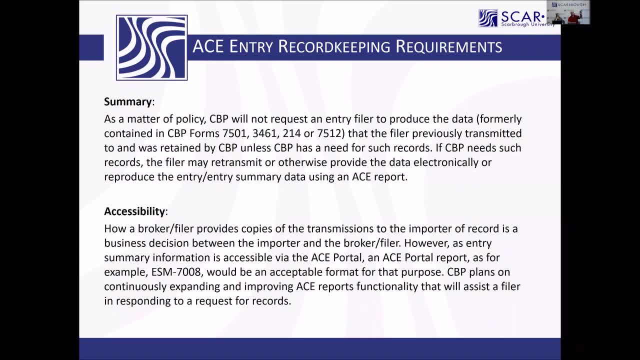 it just has fewer data elements. Okay, So that's the difference. But if say there's something complex with your shipments, you could do a 3461.. I'll give you a great example. I used to handle a lot of air freight inbound from Mexico years ago, back when Ford was building. 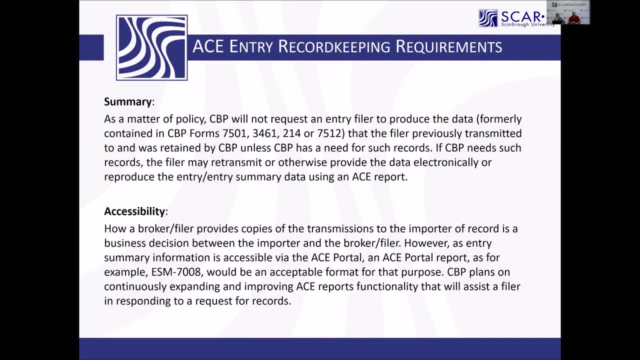 their escape And those kinds of things. those radios would come in and I would just do a 3461 to customs in the middle of the night And then the next day I would come, and then I've got 10 days to do the 7501 and pay my duties. 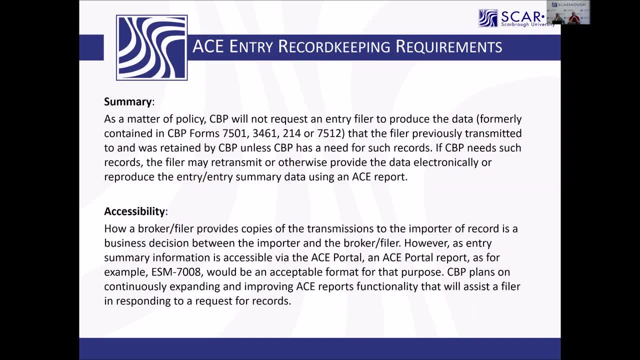 So the 3461 is first and then the 7501 is after that. Okay So, and it's got all of the details as it relates to full duties and taxes and things like that that you actually have to pay. So it's just two forms. 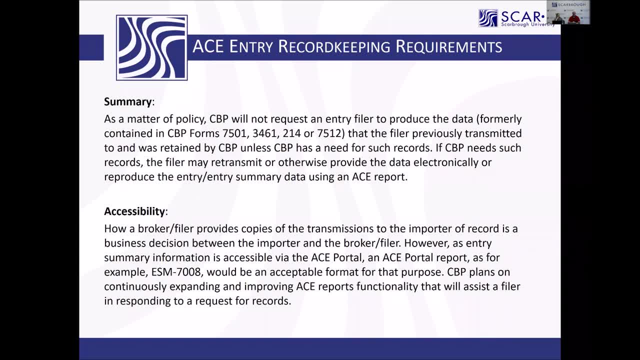 But again, both of those forms, technically, are going away and you would be able to view them in your ACE reports, And we're giving a workshop on ACE in Omaha tomorrow as well. Next country of origin. What are we doing? on time, I'm slow. 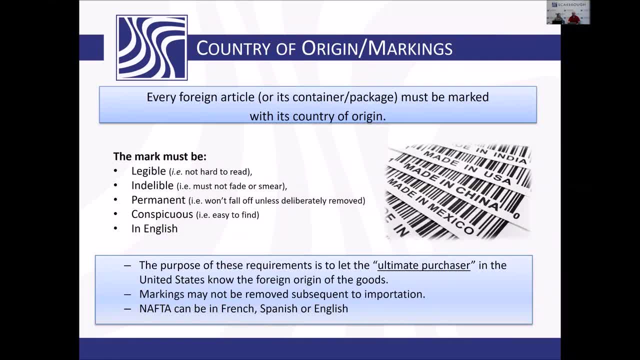 I think that if we need to run a little bit over, we can, because it's going to be recorded and we'll send it out to you guys. That way we'd get to your guys' questions. Okay, Country of origin markings. Every product coming into the United States must be marked with a country of origin. that 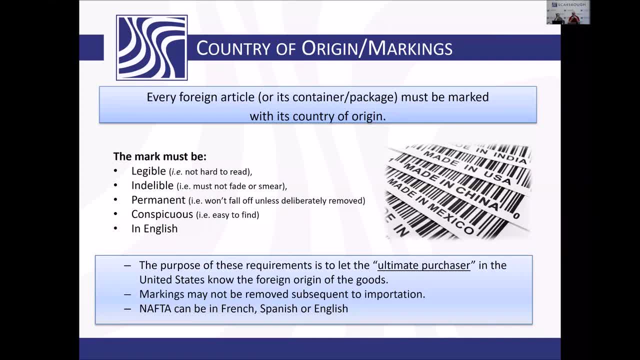 is legible, indelible, permanent, conspicuous and in English, so that the ultimate purchaser in the United States knows the origin of the goods. The reason is that, Supposedly, we care what the origin is when we're buying a product, that we care if it's. 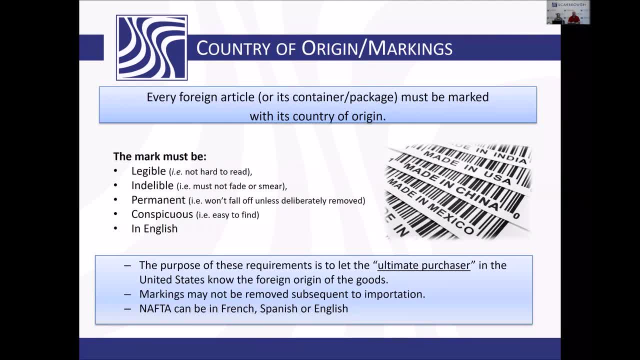 made in the USA if it's made in Germany, made in China, made in Taiwan, and so forth. So the first thing we have to do as it relates to origin and origin markings is one: determine who's the ultimate purchaser. 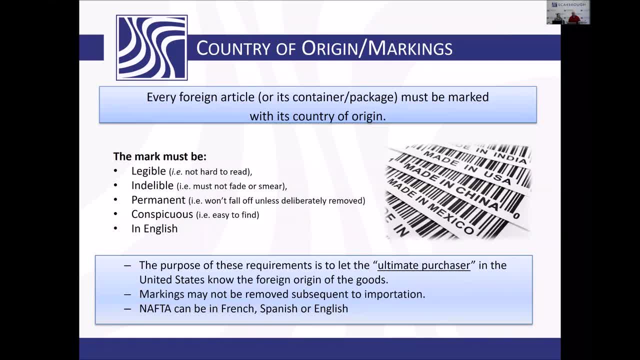 Because if the ultimate purchaser is a manufacturing company and they're going to manufacture that good into something else, then the good might only need to be required on the outside of the box. If it's going to be an end component, that's to someone buying it off the shelf like me. 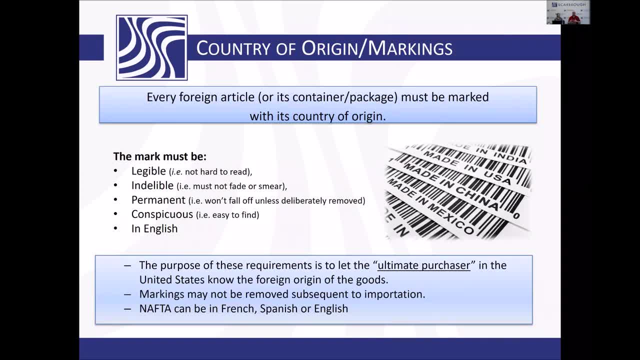 then that country of origin has to be on the product at that level. So we have to determine who the ultimate purchaser is and what they're going to be doing with it before we can determine exactly how it's to be marked. But in general it must be marked so that all of those requirements are made. 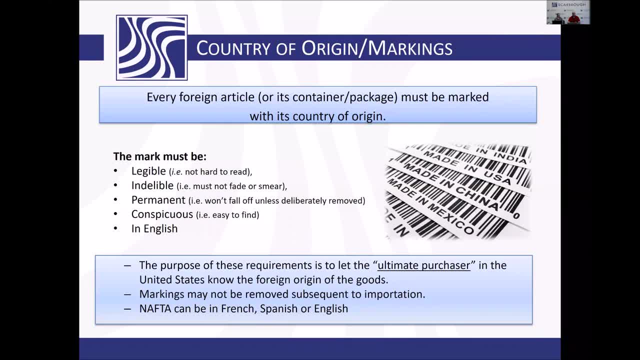 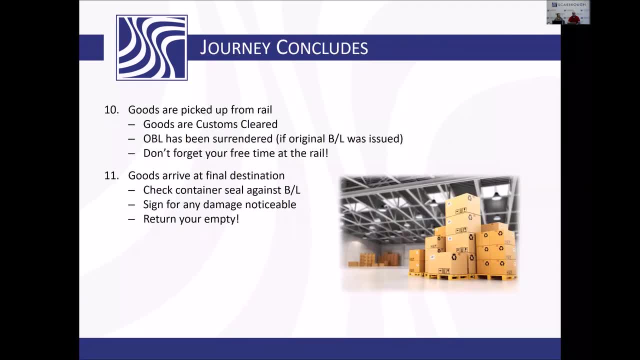 We do a lot of analysis on that too. So if we have to come look at products to determine if they're marked correctly, we can do customizing, We can do custom rulings and request that as well. So, lastly, we're getting to the end here and goods are picked up from the rail. they're 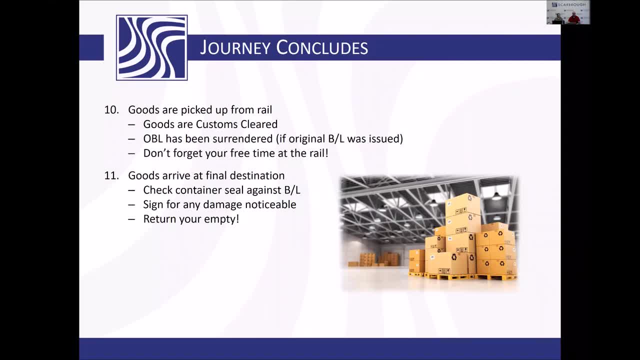 getting picked up from the truck, whatever it means They've cleared customs. They can't typically be delivered until they've cleared customs. They can't be distributed until they've cleared FDA or partner government agencies as well. The original bill of lading was tendered on the goods to the steamship lines. 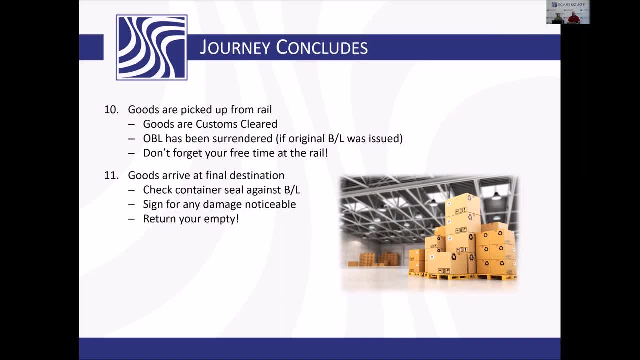 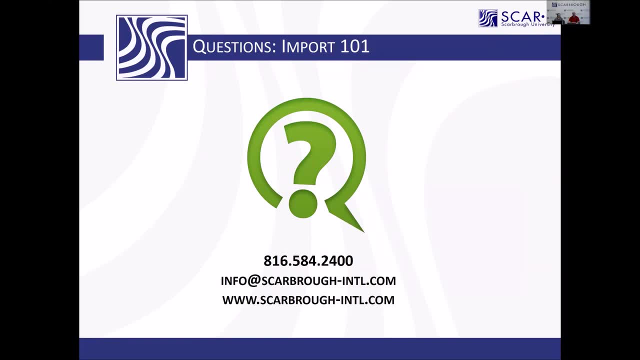 And so forth And then they get sent to the end destination. So let's go through any other questions that you have. but that's kind of a quick run-through of the 101.. Again, the compliance areas you need to be worried about are evaluation, record keeping. 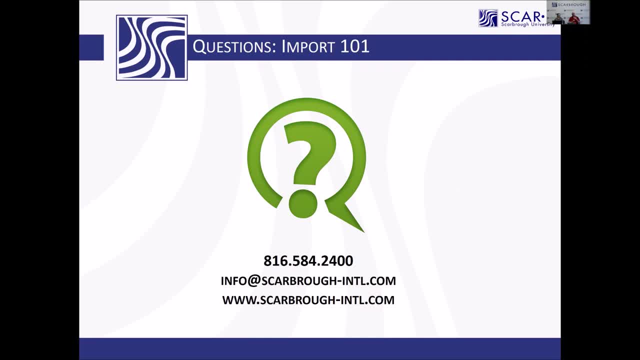 quantity, classification and country of origin markings. Those are the big five and we covered four of those today. We didn't cover quantity because quantity is really your receiving report. Did you receive the exact number that was on the packing list and invoice? 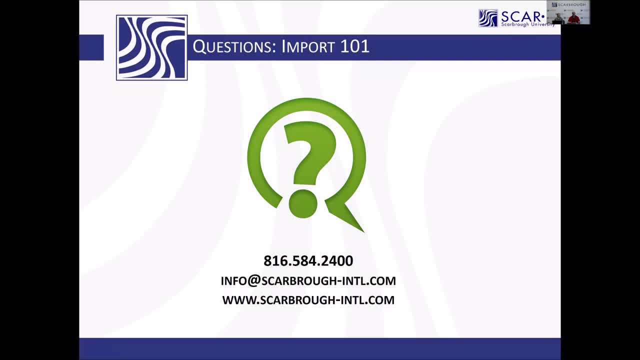 If you didn't, do you have processes and procedures in place to notify the customs broker of what was actually received and report it to customs and make sure that that gets corrected, Because if you receive too many of a product, then you owe additional duties. 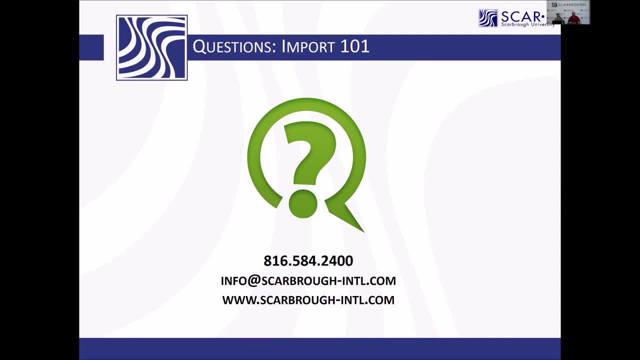 If you receive less of a product, then you want to get a new one. You want to pay less duties, So, anyways, quantity is again. that's one where customs comes in and just matches documents reported, so you're receiving reports. 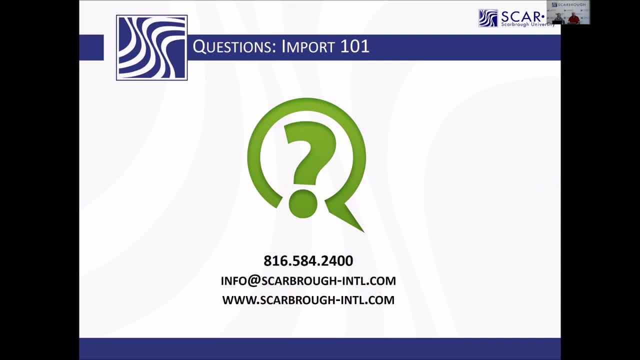 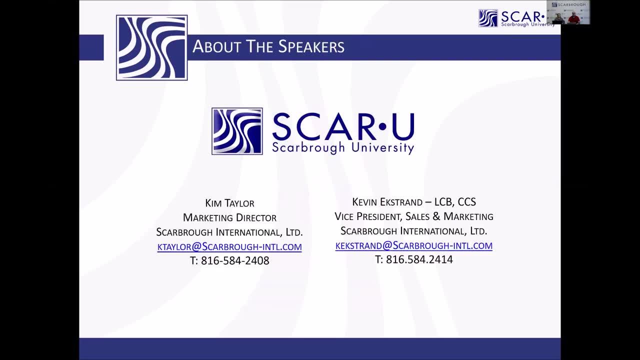 Make sure that you've actually received exactly the right amount So that one's pretty easy to speak about. Okay, so, as I mentioned, we will be sending out a copy of this presentation. We have either the full training that we send out a link to that, and we also have this. 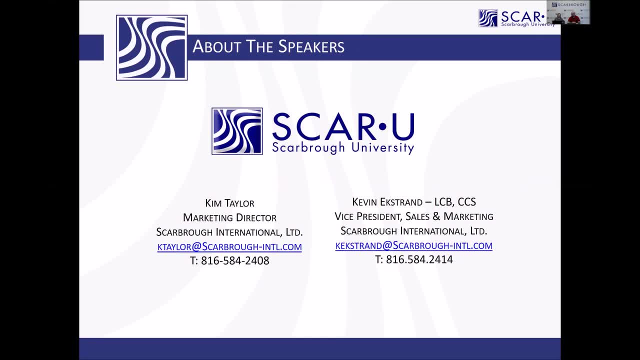 split up by questions. So if you have a question and answers that we put out on our YouTube page, I highly recommend you guys subscribe to our YouTube page. We've got a lot of training out there. You guys are welcome to it, It's free and it's out there in the public, so share it with all your people. 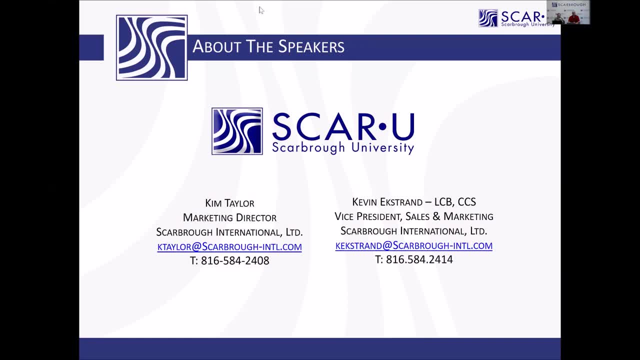 One question that just came through: can we assist shippers or importers with determining HTS codes? Yes, We do it all day long and again, that's an intense process where we're trying to get all the information out there. We're going to look at products. 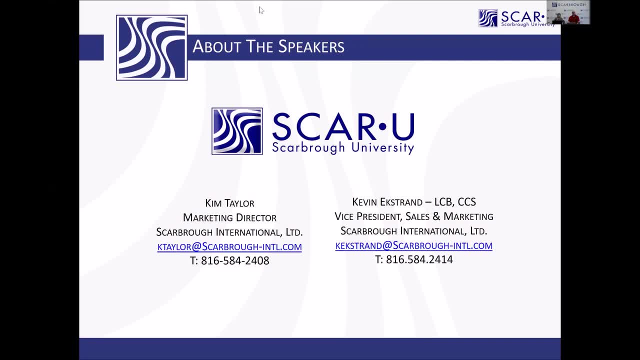 We're going to look at marketing of products to see how it's being distributed, And the reason I say marketing is because there's a lot of use provisions. I live here in the Midwest and we have a lot of agricultural equipment, a lot of ag products. 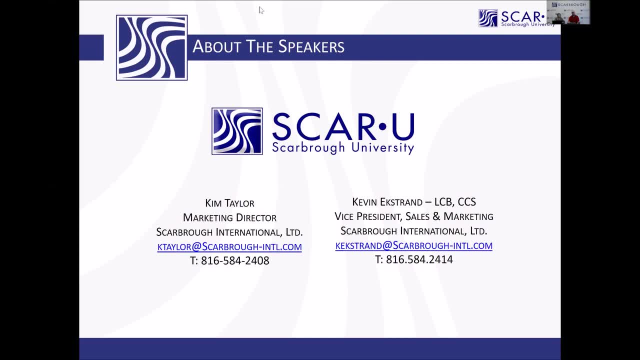 And agriculture typically has some additional tariff numbers that allow things to come in maybe cheaper or free of duty because of the nature of the product, And so we always want to look at the exact product, what it's made out of, how it's being. 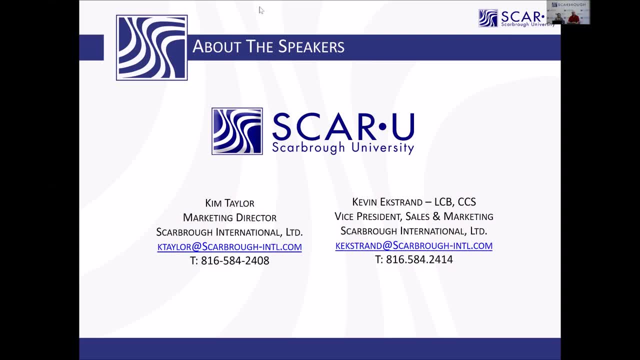 used. how is it being marketed for use? in order to come up with that HTS number for you, But it can be a very time consuming process. We're also going to look at customs rulings and things like that, but that is a service. 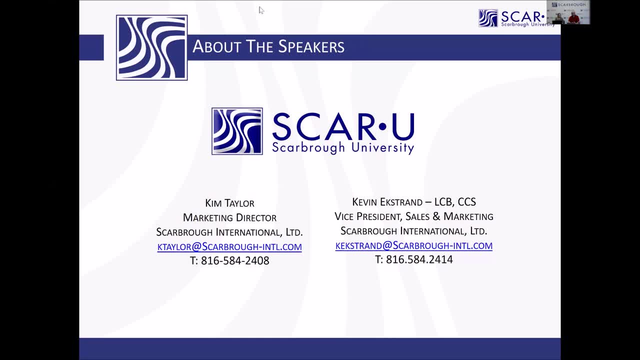 that we provide Awesome. Another question that came across is if we can get into the Incoterms some more, And I know that Kevin mentioned that there can be an entire half day training on Incoterms. We actually do have a link out there on our YouTube channel for Incotermscom. 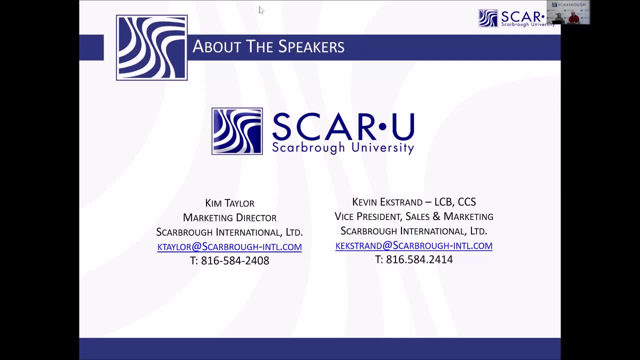 There's training that you can go and check out. You'll get a link to that with the follow-up email. If you have specific questions or you want us to help guide you on which Incoterms to buy on- or sell on, for that matter- definitely contact us directly and we can help you with. 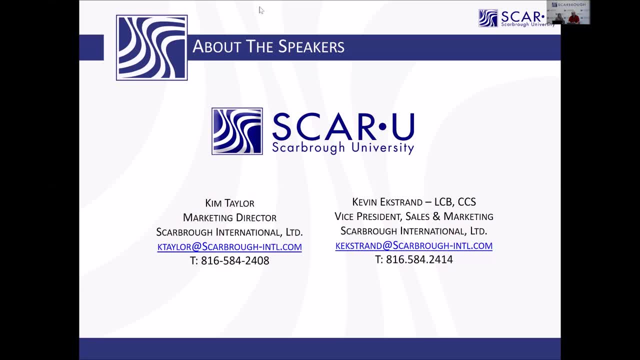 that. Another question in here, a good one- is: can a supplier change importing terms prior to a new shipment without the wholesaler's permission or knowledge? You know, there's- Yeah, Yeah, There's nothing in customs regulations that That's really the contractual obligation between you, the buyer, and your seller overseas. 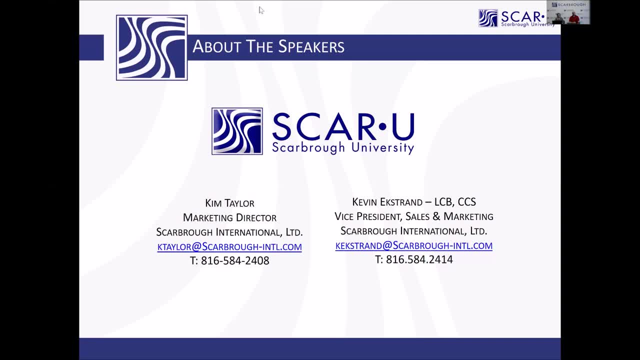 And there's nothing regulated on the customs side of things that can prevent that and or that allows that. So it's really outside of the purview of customs in general. I wouldn't think that you would want them to again, my recommendation is you as a buyer. 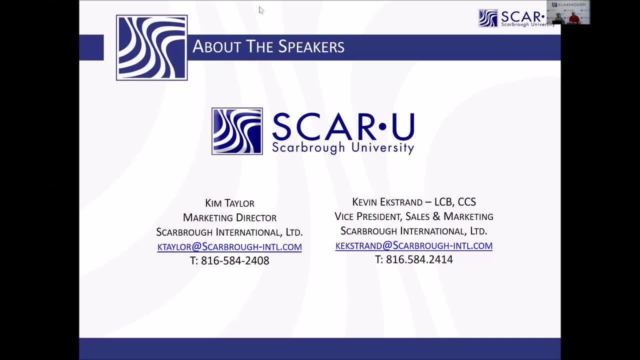 take control of the Of the Incoterms. buy on an F-term. if it's ocean, buy FOB. but use that F-term, Even that E-term Ex Works. Ex Works is a good term to use, especially on the import. 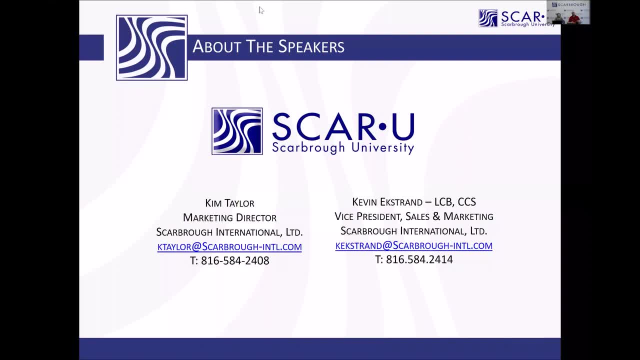 side. The only thing with Ex Works is that it requires that you pay for any export formalities in the country. Now, that's not bad in Europe, because they don't have those types of that many conflicting terms. Ex Works is very common meaning: I'm going to pay for the truck to pick it up at their 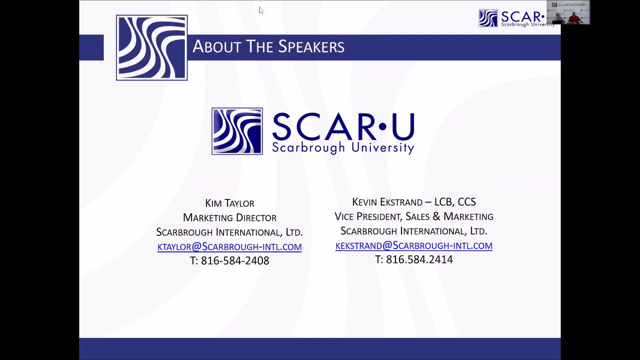 dock, deliver it to the port and ship it out- Very common in Europe But that can be really complex in some countries, In some Latin American countries. it can be very complex in Asia as well, because the cost to get, Because they require export declarations and export customs clearance and you're subject. 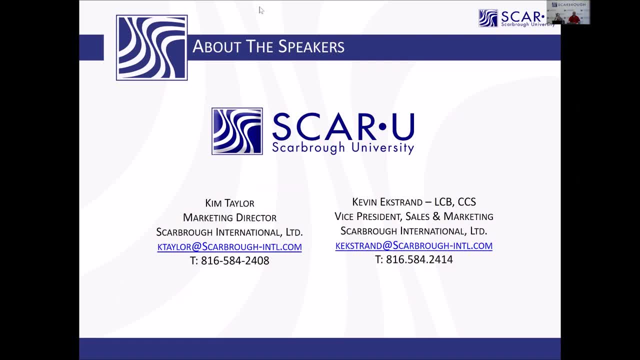 to paying those fees. And sometimes that inland fee in Asia can be really expensive if that manufacturer or supplier, If it's say way inland or up a river or whatever it might be. So that's why we recommend letting them handle what's on their side at an FOB. 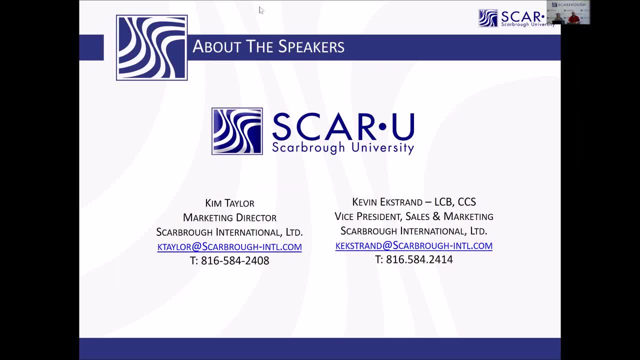 Let them take care of paying for and scheduling the shipment and paying for their charges at the origin location and you take it from there. That's why we recommend the F-term. But E is not bad. You just have to be very, very particular with what country we pick from. 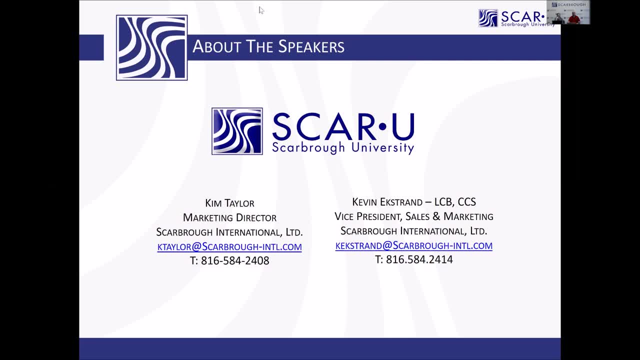 The reason I don't like C-terms as it relates to equal terms, is because We're using their freight forwarder and you, as the importer, who's responsible for the security filing, might not know the shipment is being sent because you don't have great. 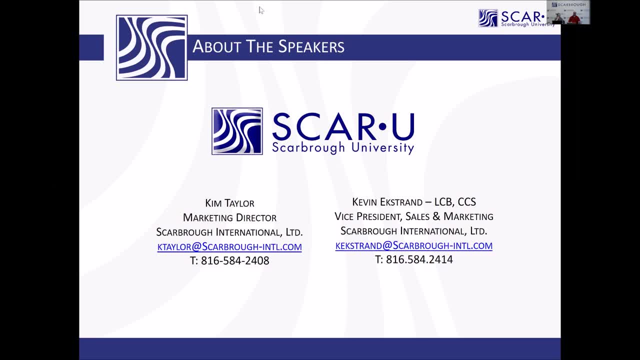 communication with their freight forwarder, especially if that's out of Asia, where they change freight forwarders very, very often in order to maximize their return and profit on the freight piece. So, anyways, that's why I don't recommend C-terms, is you lose control, you lose visibility. 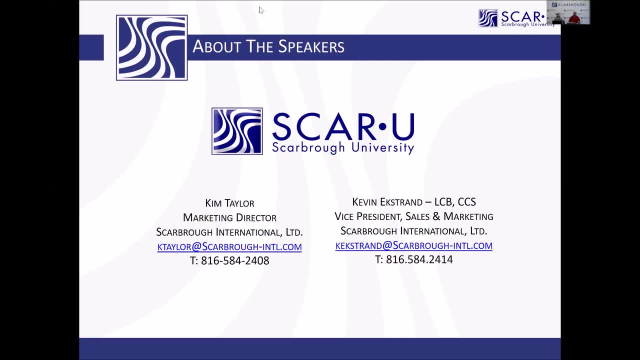 and then you're at risk of a potential violation for the import security filing not being on time. Very perfect. In regards to the HTS tariff code, again, can that be a different code from the exporting country and the United States? Yes, In the United States and I've talked to customs inspectors. my office years ago used to be. 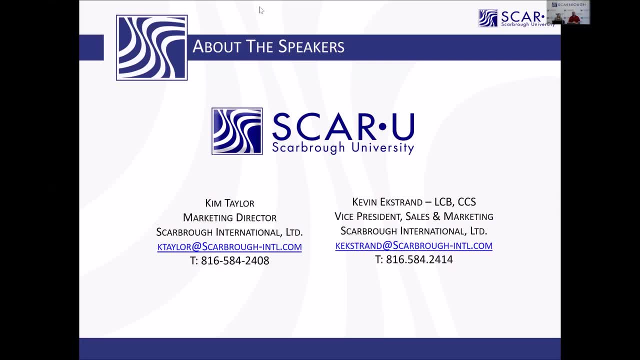 right next to customs inspectors and he would say: we don't care what they think the tariff number is in the foreign country. And we see that. We see that a lot in Asia And honestly, some countries have ruling systems and their opinions from one country to the. 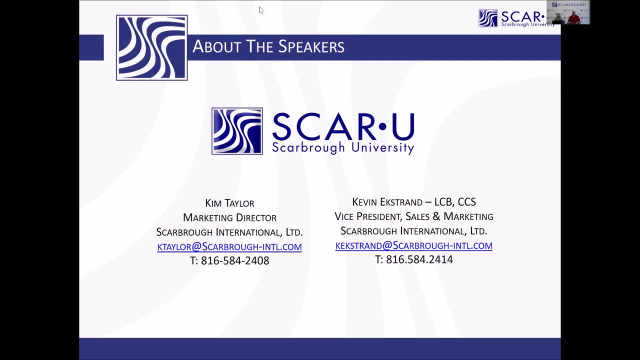 next vary. So I'll give you an example. I had a client that had a binding ruling in the United States for a particular product. Canada had a binding ruling for the same product and they were in completely different areas. One was a power supply, one was a battery. 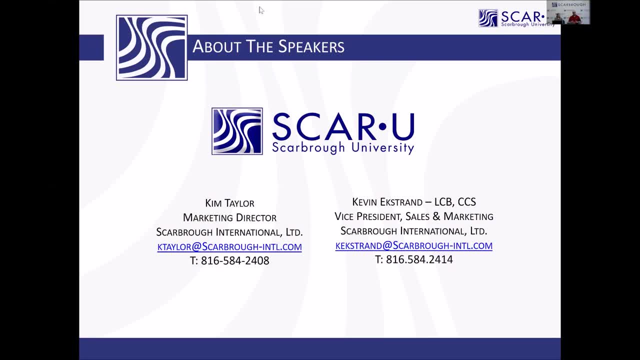 And again two customs rulings, Two different HTS numbers, And that's very common In Asia. they like to pick the tariff number that gets them the maximum rebate. That doesn't mean it's right here. So my advice to you is: don't listen to them on their tariff number. 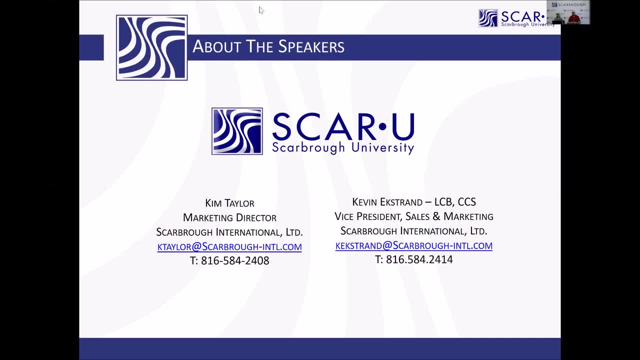 You do your due diligence and you make sure it's right, Because when we declare or make a declaration to US customs here in the United States, we want to make sure that that tariff number is absolutely 100% correct for you. 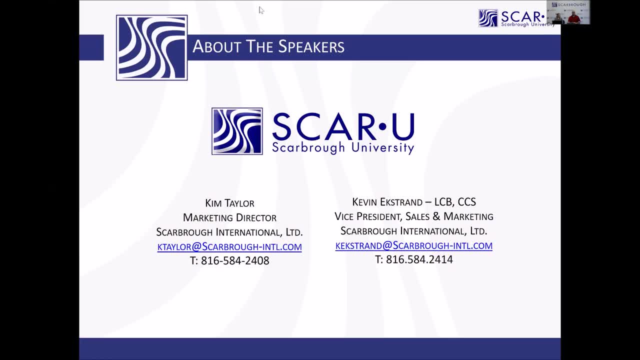 You want to make sure it's correct for you. It has zero effect On the shipper overseas. So if it comes in with the wrong one, you know, tell them not to include it, but make sure your broker declares that correct HTS number based on the product here in the US. 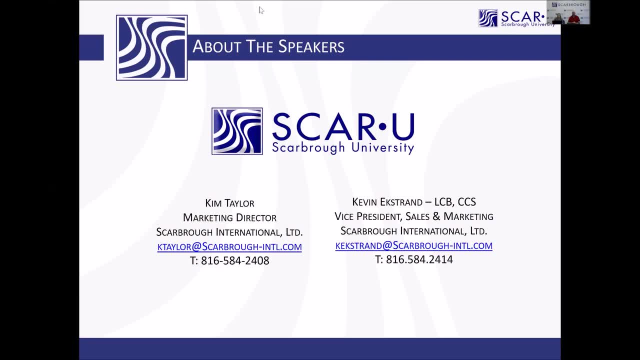 and you're protected. Okay, let's go back to the 7501.. You had mentioned matching up what was received to what shows on the commercial invoice, But sometimes we see shipments- ocean shipments- come in much after the 7501 entry date meaning. 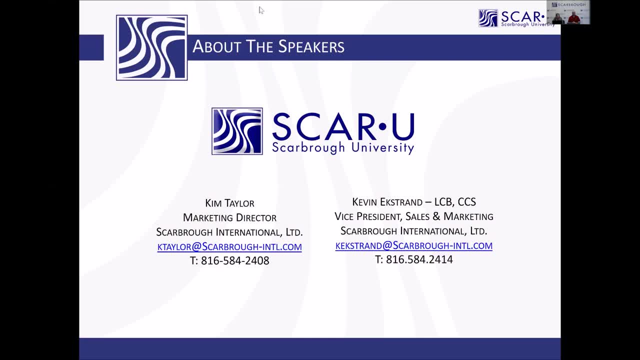 post-entry is required to correct the 7501.. Okay, So if the quantities are incorrect, is this okay? It is okay And one of the things that we have to think about when it comes to post-summary corrections and that, again, if the receiving report doesn't match what's on the 7501, then you need to. 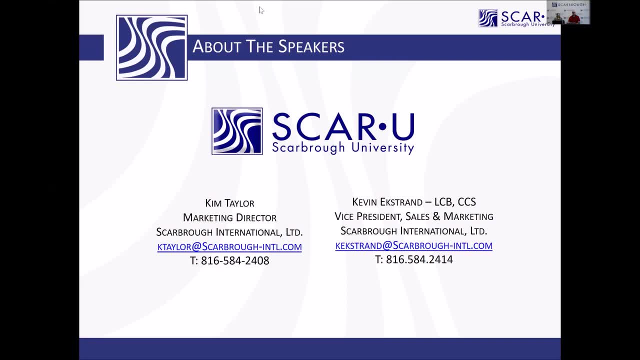 make a post-summary correction. ACE has made that easier, But we also need to look at the de minimis rules and see, if it does need to, how it needs to be reported based on the change in duties. Usually that's what we do. 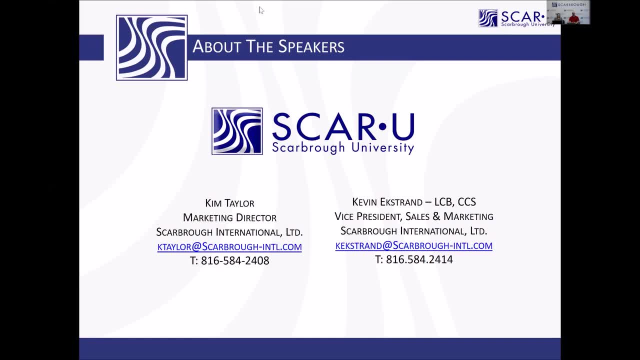 Usually there's a $20 change there, So we would want to look at the de minimis to see how we would handle it specifically. But you would definitely want to keep that record and make sure that you communicate well with your customs broker any changes between the documents and what was actually. 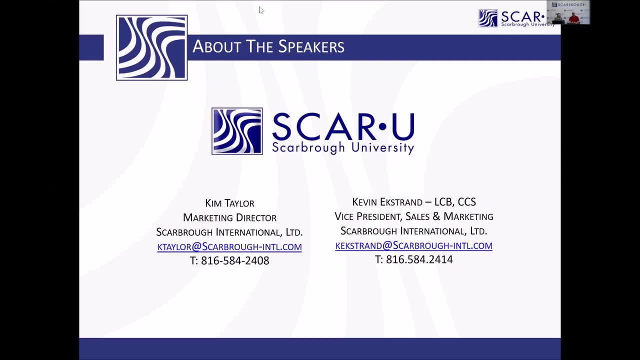 received, Put in good processes and make sure that communication flows between the person receiving it and the person communicating with the customs broker. if they're different, Well, I think we've got one more question. that's live out here. Some other people have submitted questions. 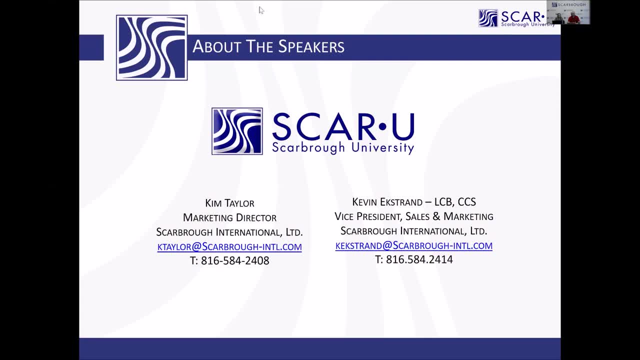 Prior to registering for the webinar. we will get back to you guys directly. This one last question that's out here is: are there minimum invoice requirements that are required for US Customs? There are specific invoice requirements that are required on every single customs entry. 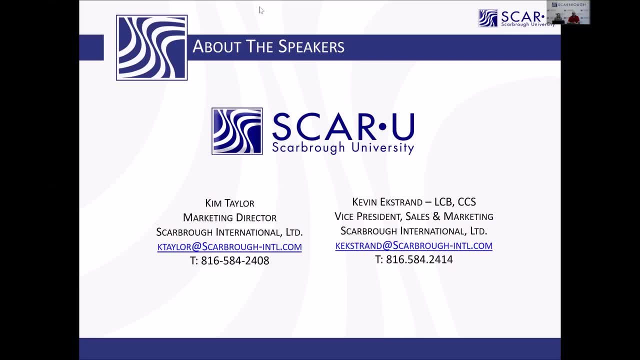 And I can send you what that list is And that list is actually in 19 CFR- the Customs Regulations. And I can send you what that list is And that list is actually in 19 CFR- the Customs Regulations. And that list is actually in 19 CFR- the Customs Regulations. 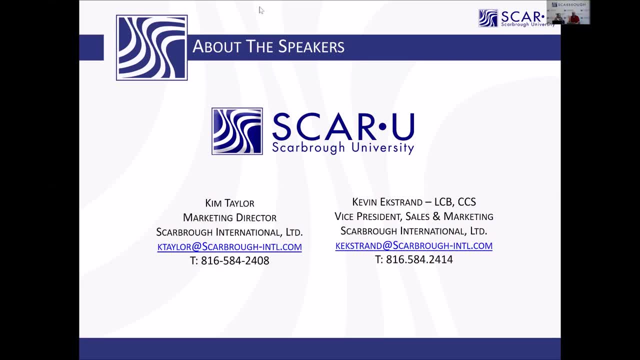 It has what the specific invoice requirements are. Now, you have to be mindful that some of those requirements might relate to specific government agencies and things like that. That might not be specific to your product, But there are specific customs requirements that are out there. 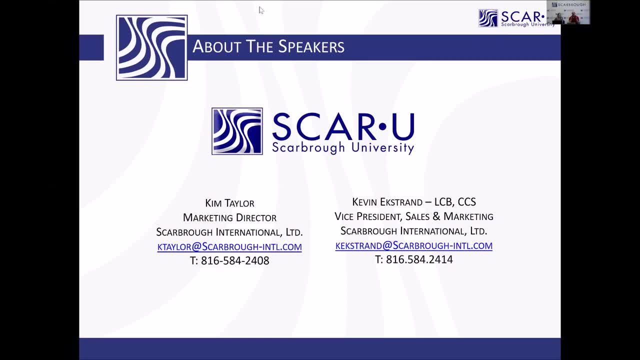 There's a list. I can't remember how many was on it, but I do have that list And I'm happy to send it to you And we can post that out there with this presentation on our website as well. Okay, live. 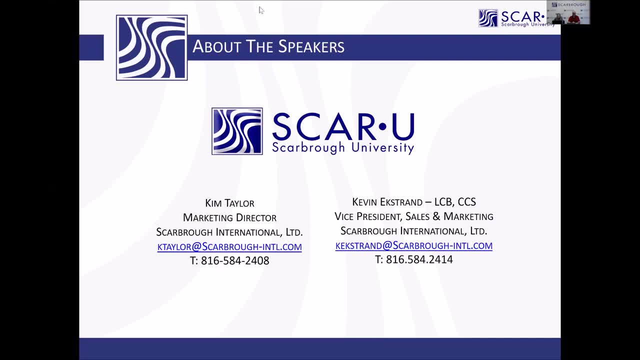 Let's just do one more question. okay, if our supplier sends us items at no charge, can they be listed on a commercial invoice and clear customs at zero dollars? or does every item need to have a value? the answer is no, they can. they cannot have a zero value every. 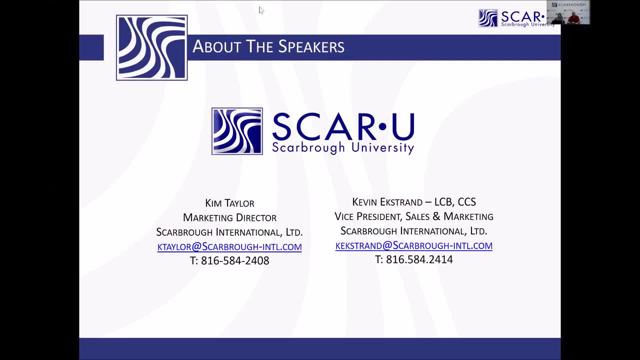 product that you would want to import has a value. it has a value for insurance purposes. maybe you didn't pay for it. and again, when we're looking at this, we're looking at what it is, we're looking at those different degrees of. are those five different elements of valuation? the number one is transaction value, and we 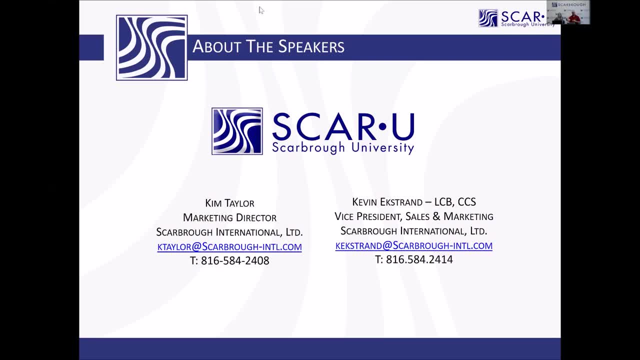 talked about that one today. so when you're not having a transaction where you've paid for a product and they're giving you a product for a small fee or for free in this instance- then we go down to the next level, and that one is value of identical merchandise transaction value of identical 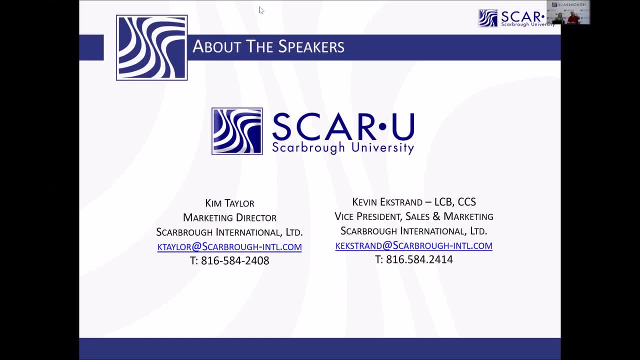 merchandise. you're looking at what it is. we're looking at those different degrees of so. in that situation where we can't value the product because you didn't pay for it, you don't have the unit price, we would look at what is the cost of that. 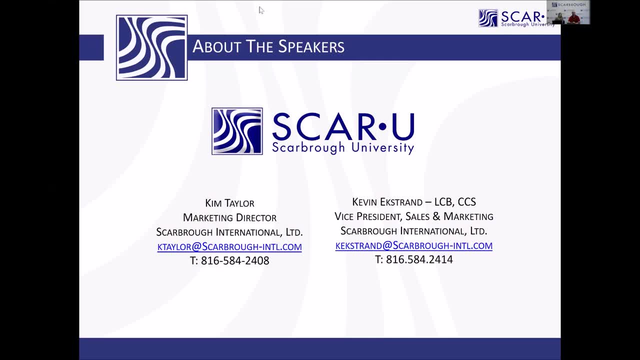 product that you didn't pay for. and we see that a lot say you bought. see, you bought a bunch of these cups and you bought a hundred of them at ten dollars apiece and then, because you bought a hundred of them at ten dollars apiece, they give you ten of them for free. I know that I would just utilize the value. 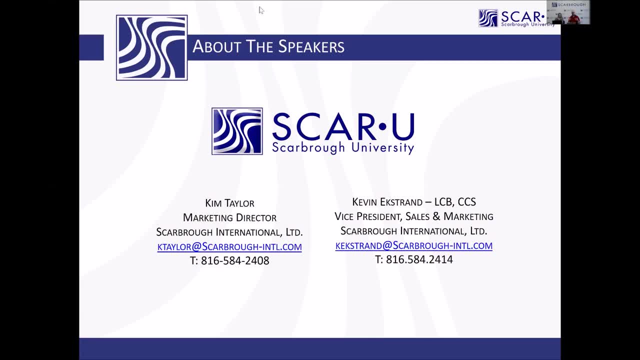 of the price of one of these products that you've purchased, because that's an identical product that you did have a transaction value with. so that's the price that would need to be declared, because it does have value, has value for insurance purposes and it has value for customs purposes. it will never be free. 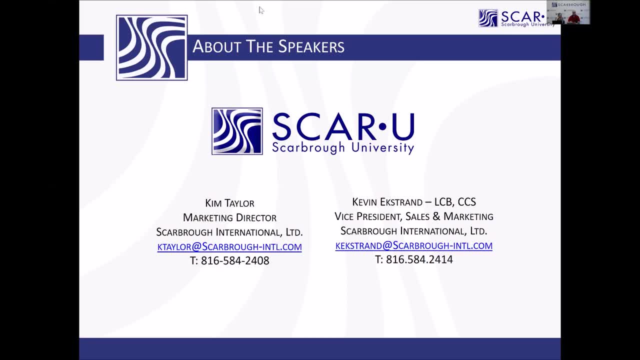 nobody ships anything for I mean that's provides that that has no value whatsoever. so, anyways, that's the value we've utilized. that can become very, very difficult, but again, we look at. we look at each of the different ways to value a product in order to determine. 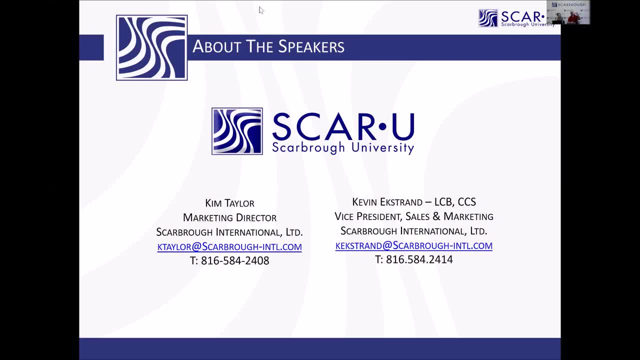 the right one. so we've got identical merchandise, we've got transaction value of similar merchandise, we've got computed value, and now I'm losing, losing it here, but and then? so anyways that we would find a way to come up with the correct value. but you, you can bring it in. it can show free of charge meaning. 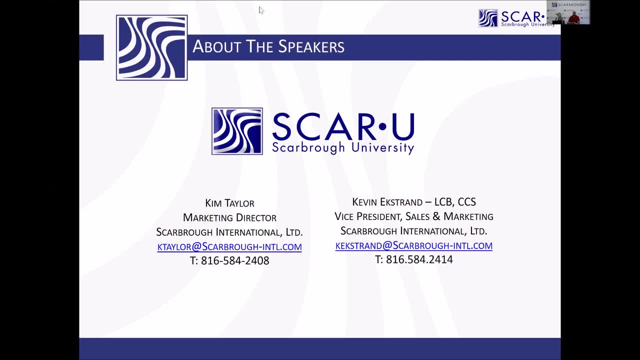 you didn't pay for it and that's good for accounting purposes. and if customs comes to audit you for valuation, you can say, no, this is what I pay. I receive these for free, but I did declare the correct value to customs in order for duty for payment purposes, so that wouldn't that would come through. I. 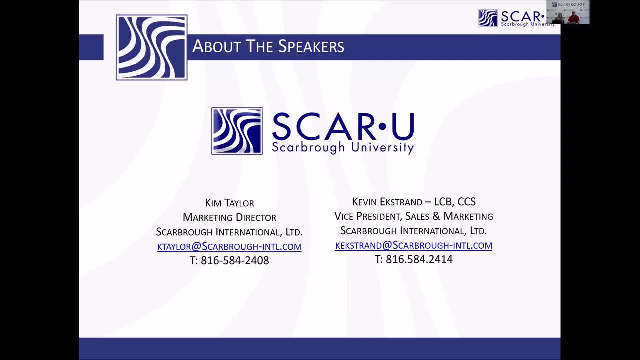 hope that helps. and we do have a couple other questions in regards to, let's say, duty drawback for example. we have a whole nother training on that. so your duty drawback questions, definitely send us an email and we can help you through that. anybody that's out there asking about our processes for best practice or 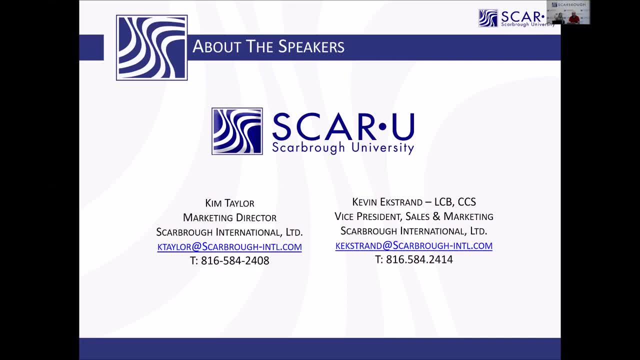 auditing. definitely talk to us. like I said, we're very known for our trade compliance consulting. that's something that we can talk to you about, something we do every day. newer regulations that are out there- those are just different news items that we continually post out on our newsletter as well as our blog. so